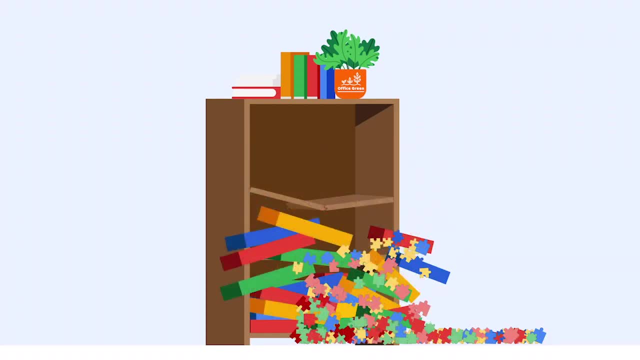 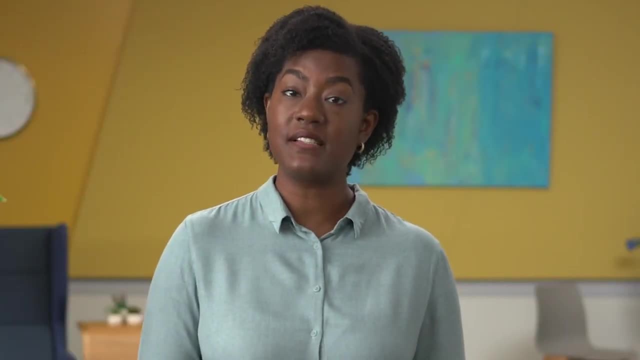 different puzzles. One day, a shelf breaks and all the boxes topple over, scattering the puzzle pieces everywhere. To get each puzzle organized again, you need to identify the pieces that correspond to each particular puzzle, gather them together and put them back into their correct 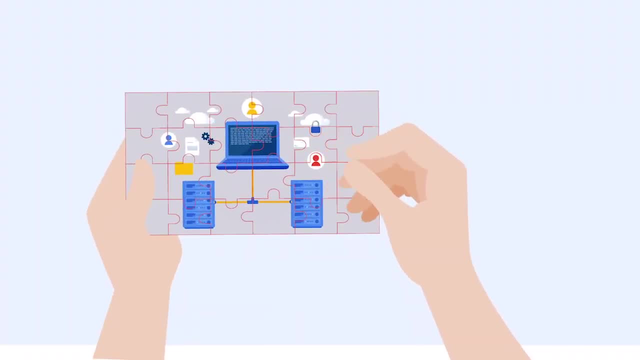 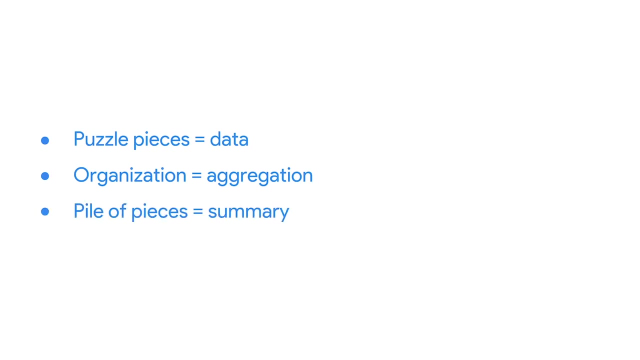 boxes. Only then can you work with these pieces and create a complete picture. So in data, the puzzle pieces represent the data that lives in different separate data sets. Getting them organized is the aggregation process. Then the piles of pieces that complete a single puzzle become your. 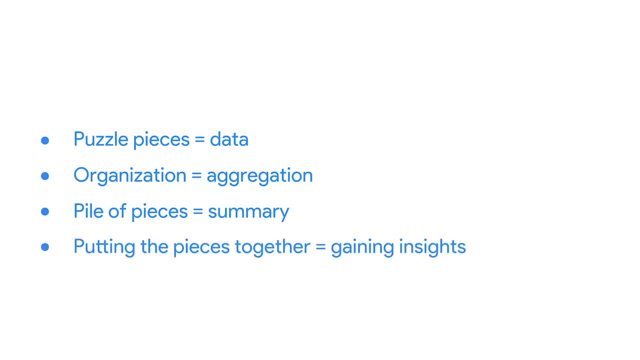 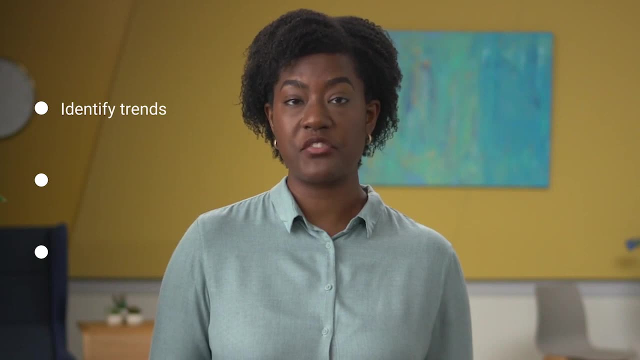 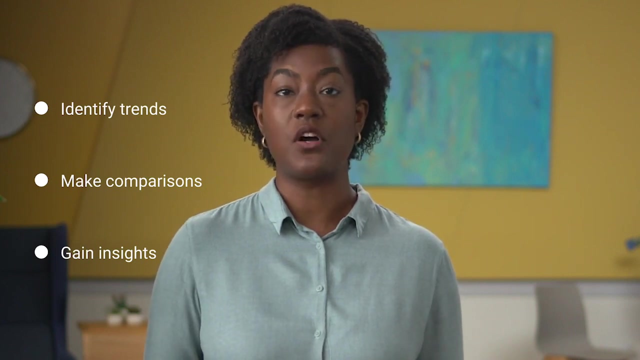 summary, And finally putting those pieces together and collecting them all together is the aggregation process. back together is like analyzing them to gain important insights. Data aggregation helps data analysts identify trends, make comparisons and gain insights that wouldn't be possible if each of the data elements were analyzed on its own. For instance, data on high school. 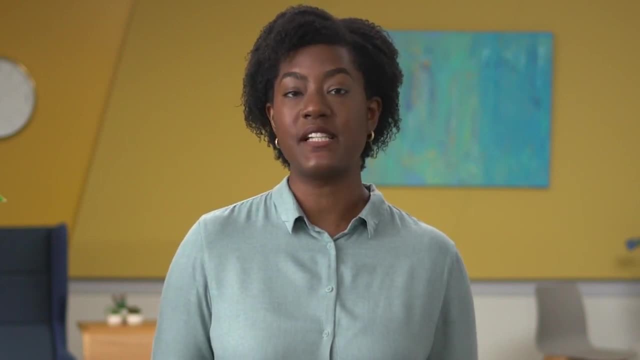 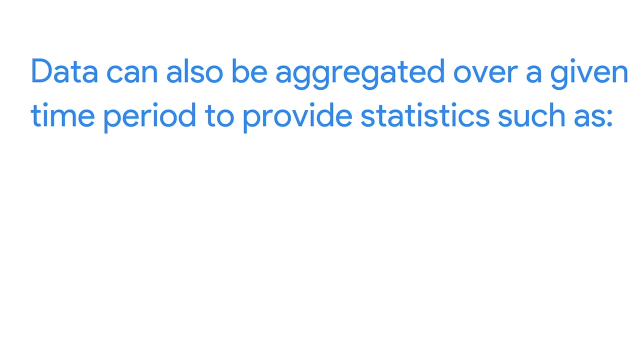 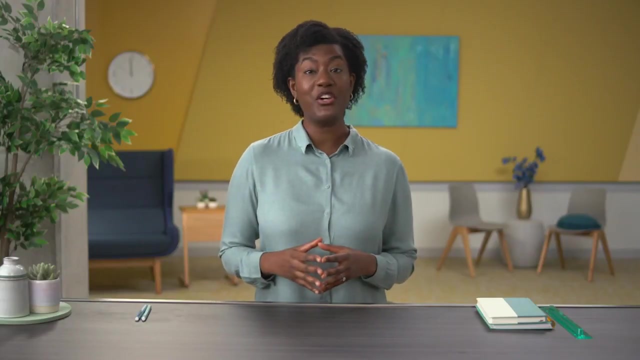 graduations for individual students can be aggregated into a single graduation rate for an entire class. Data can also be aggregated over a given time period to provide statistics such as averages, minimums, maximums and sums, For example, that same yearly graduation rate data. 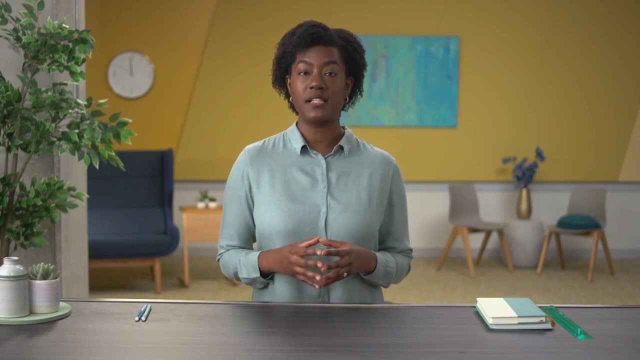 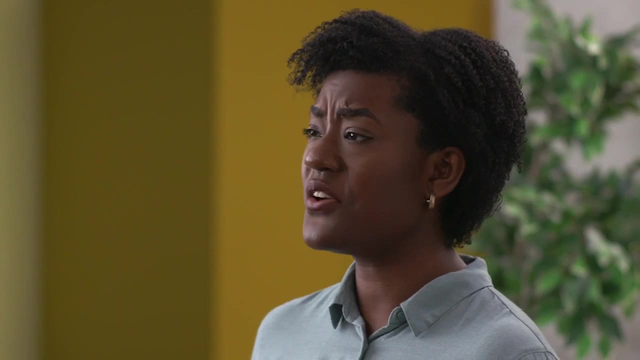 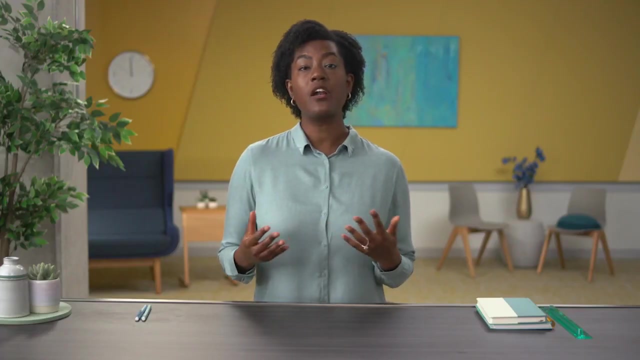 can be aggregated once again into a summary that shows us graduation rates for districts, states and countries. Here's another example. Let's say you had data on real estate sales in a particular neighborhood for each of the past 10 years. If you aggregated all of that data, 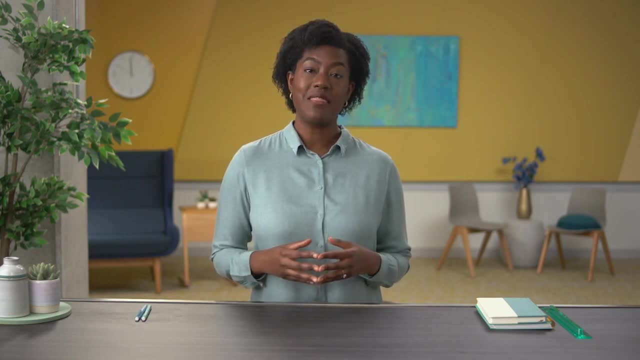 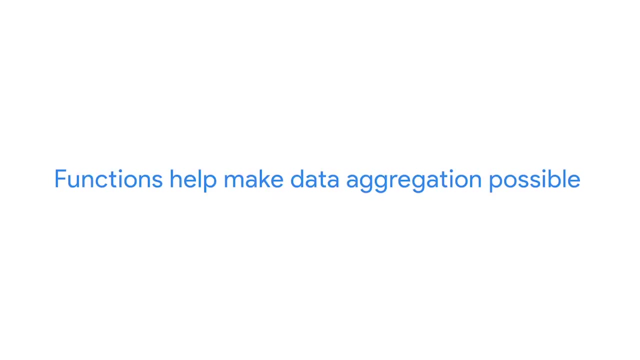 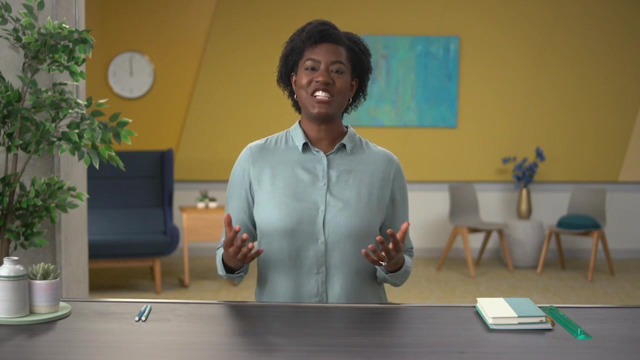 you'd be able to discover the average price of a home in that area and how values have increased or decreased over time. Functions are a big help in making data aggregation possible. You'll learn how to use some of the most common ones to create your summaries soon. In addition, we'll talk about aggregating data. 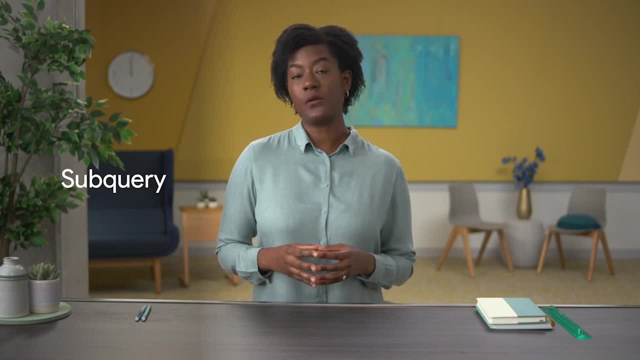 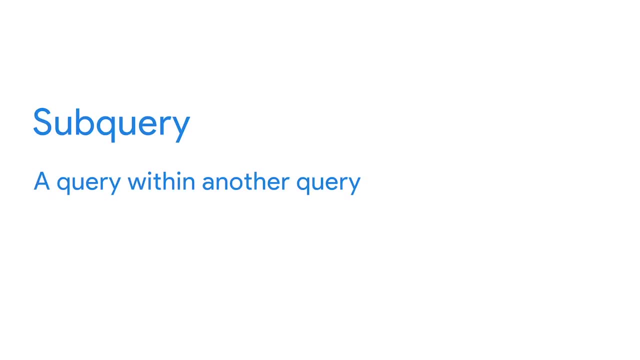 using something called a subquery. You've seen SQL in action and you understand that a query is a request for information from a database. So a subquery, also called an inner or nested query, can be aggregated to a query within another query. 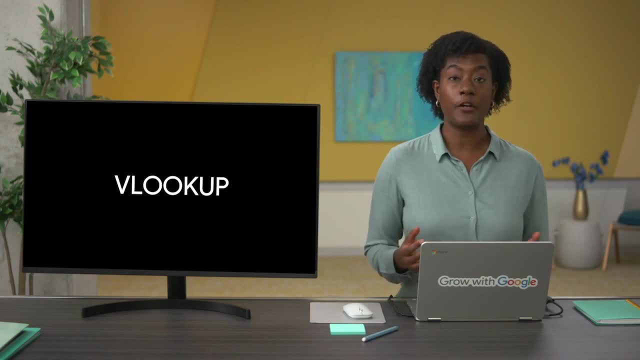 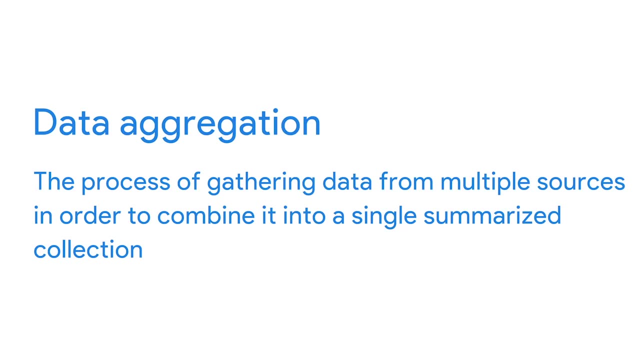 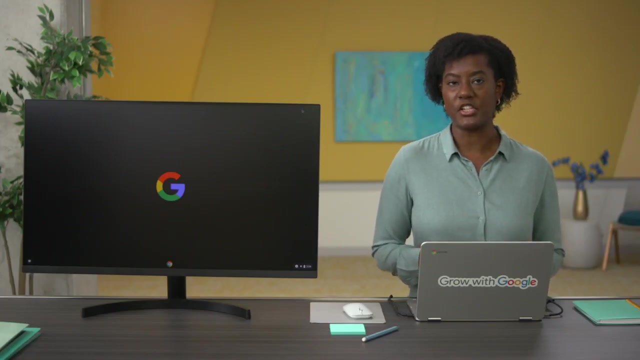 In this video, we'll prep our data for VLOOKUP, a data aggregation tool. As you learned before, data aggregation is the process of gathering data from multiple sources in order to combine it into a single summarized collection. Data aggregation can give you all kinds of information about the 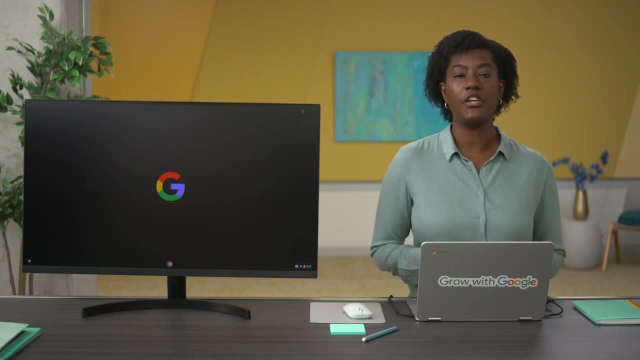 data you are looking at. For example, in marketing, you can aggregate data from an ad campaign to see how it performed over time and for particular customers. Travel companies use data aggregation to figure out how much their competitors charge for a certain flight hotel. 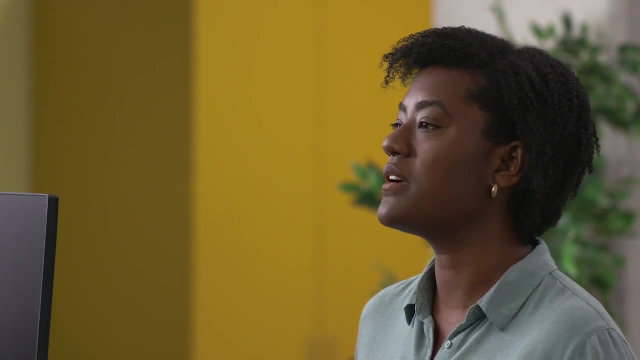 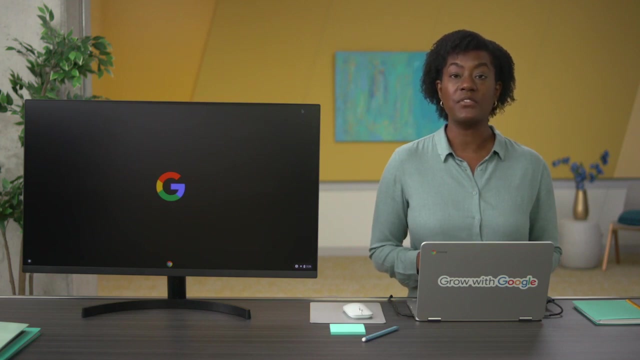 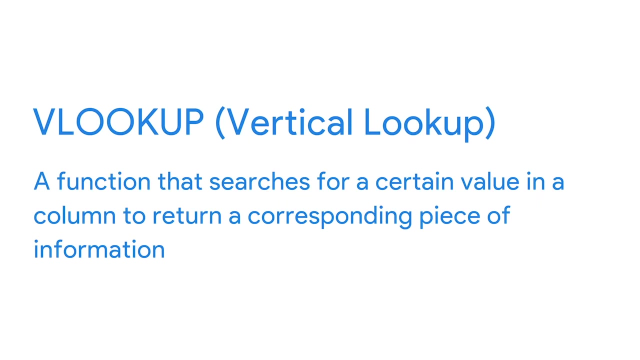 room or rental car type. Then they can make sure they price their own products as competitively as possible. One thing these businesses all have in common is that they can use VLOOKUP to help them achieve these goals. As a reminder, VLOOKUP stands for vertical lookup. Basically, it's a. 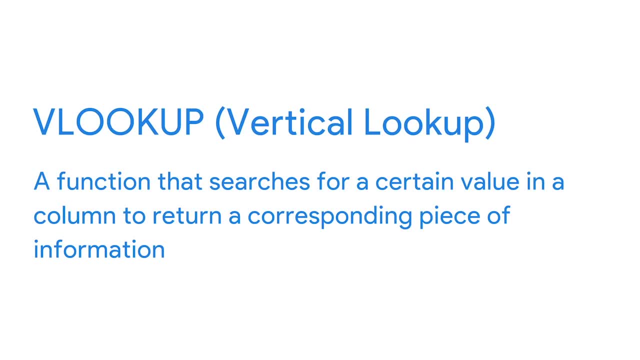 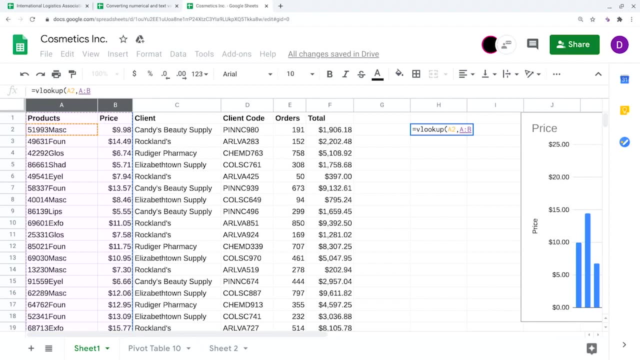 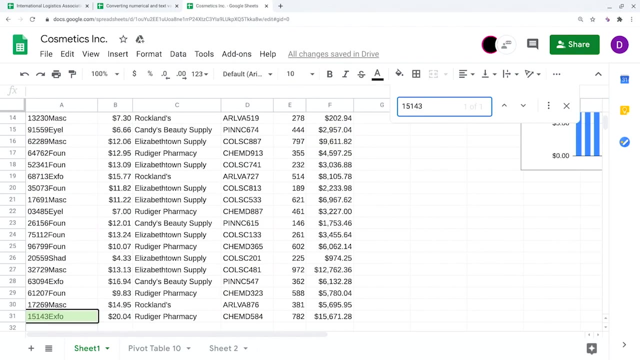 function that searches for a certain value in a column to return a corresponding piece of information. Earlier, we used VLOOKUP to take the value in one cell and search for a match in another. We were able to match a product code made up of numbers and letters that lived in one. 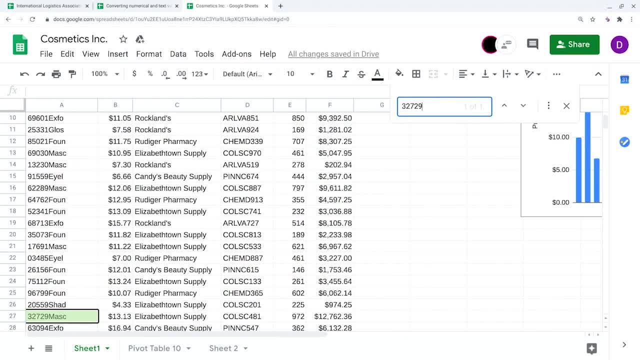 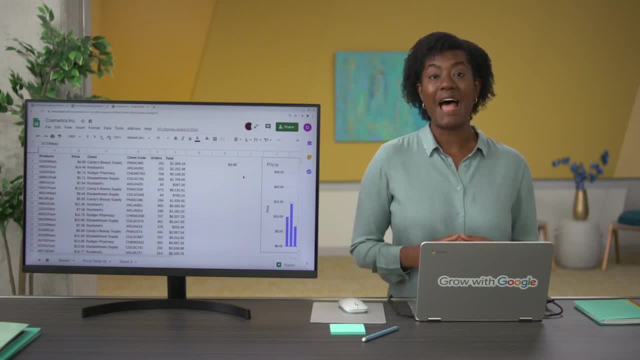 spreadsheet to the actual name of the product that lived in another. But before any of that can happen, we need to make sure our data is properly prepared. As you've heard many times, clean data is much more likely to give you accurate results. 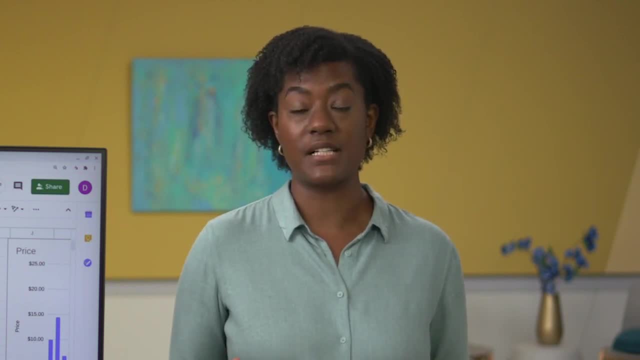 So let's start with the first common data cleaning task: different data types. For example, a dataset might have dates formatted as numbers or numbers represented as text strings instead of numeric values When data is not in a consistent format or a format that the spreadsheet application. 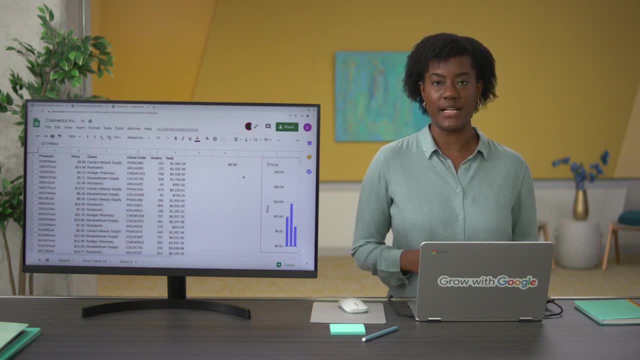 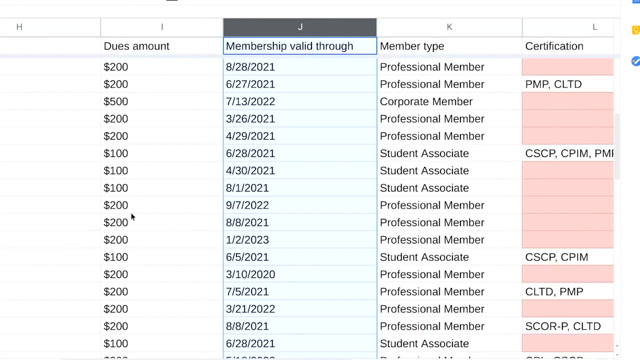 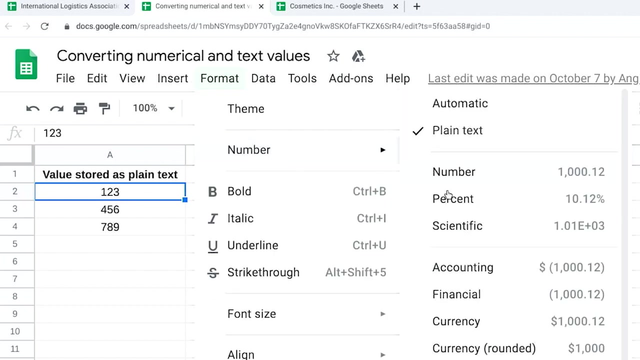 recognizes VLOOKUP, won't know what to do with that data and it'll return an error. Earlier you learned how to convert numbers to dates using the format tool, So now let's focus on converting text to numeric values. To do this, you could use the format menu to select a type of number. 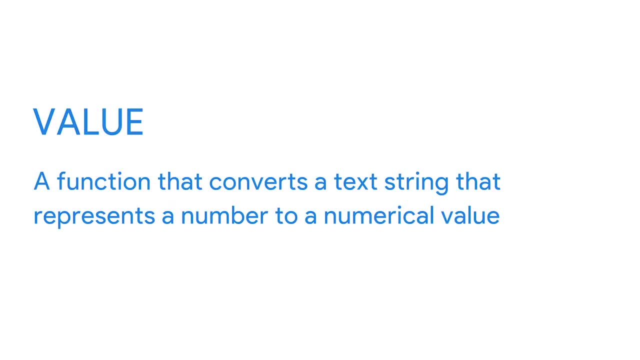 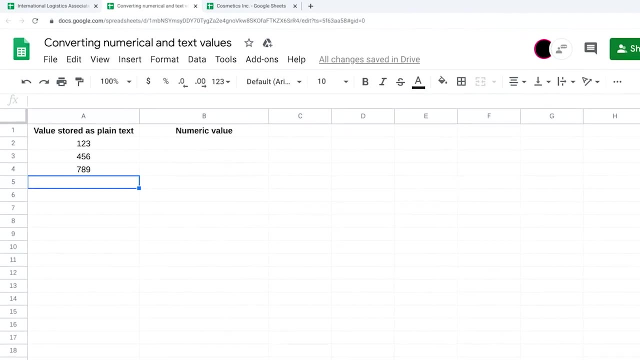 But you could also use the value function. Value is a function that converts a text string that represents a number to a numerical value. Here's an example. In this spreadsheet, the numbers in column A are currently text strings. We can confirm this by running a simple SUM function. 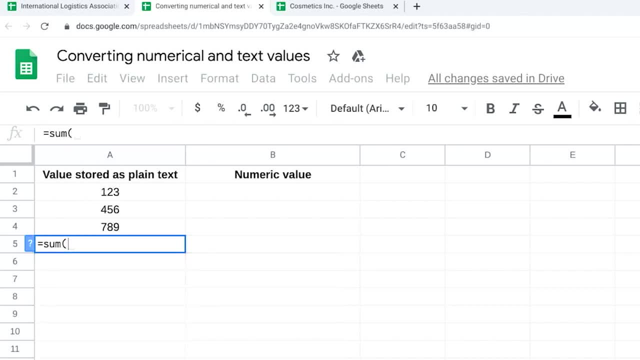 The syntax is equal to SUM. open parenthesis and then the items you want to add together. Here it's A2 to A4.. The colon says we're including everything between these two references. Now you can add a close parenthesis and press enter, or you can click and drag on the cells. 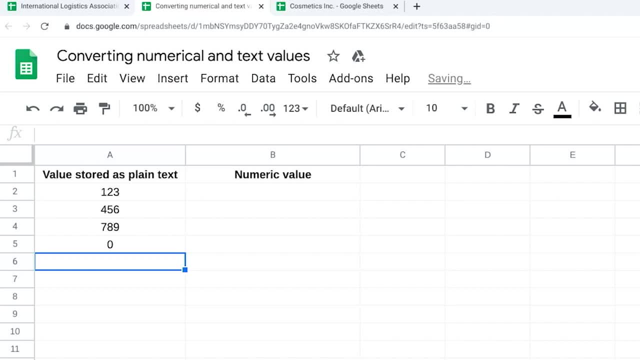 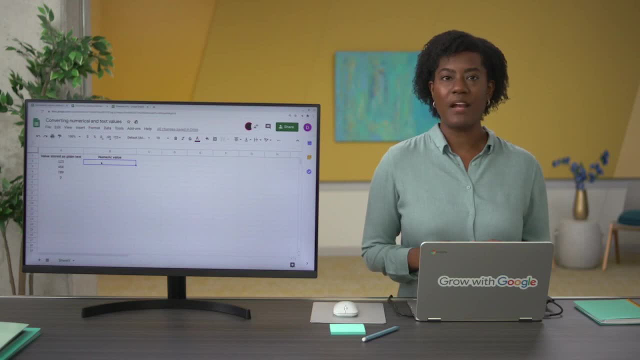 you want inside the parenthesis, to save a little bit of time. The result is zero. That's because the function doesn't work on text strings. But if we apply the value function, it automatically converts that text string to a number. So let's do this. 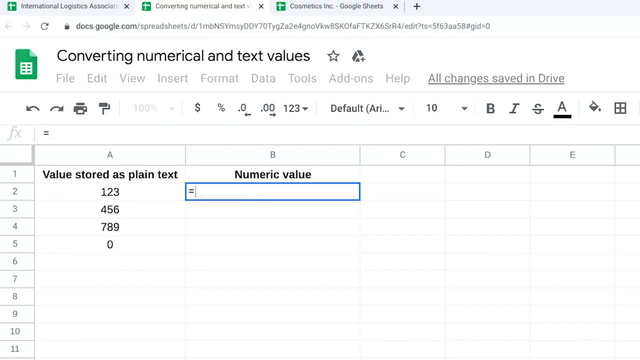 To do that we'll type equals value, then an open parenthesis. Inside we reference the cell whose value we want to convert, in this case A2.. So now, if we close the parenthesis and press enter, you'll notice that the 1,, 2,, 3 is. 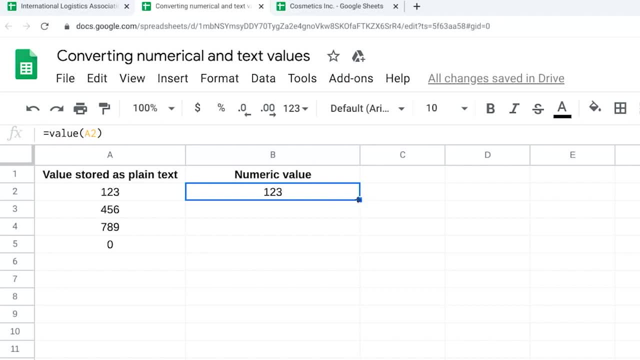 numeric. If we drag it down the column, the 4,, 5,, 6, and 7,, 8,, 9 also become numeric. Now we can test it by running another SUM function. We'll type equals SUM, Then B2, colon and B4.. 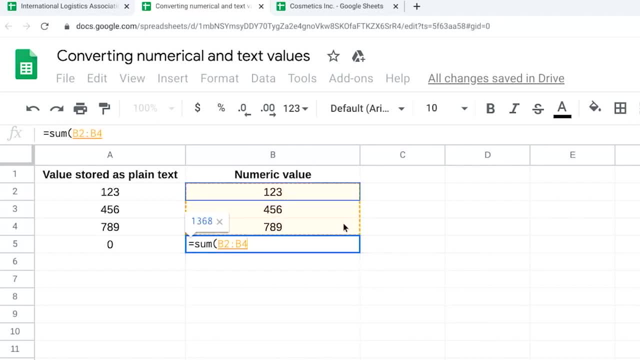 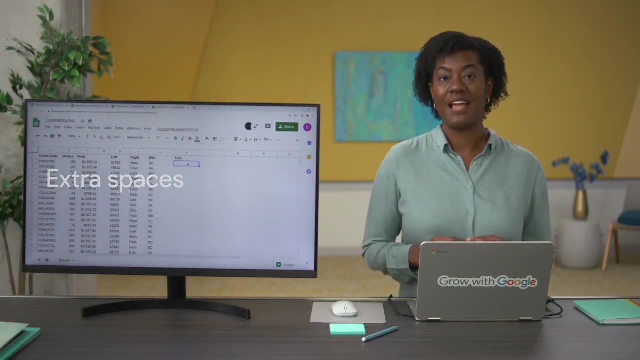 So B2,, B3, and B4 are included in the SUM, Close the parenthesis and press enter. Now it shows that the total is 1,368.. Okay, the next common error comes from having extra spaces in your spreadsheet. As you've learned, when data is copied from one source to another, sometimes a few leading. 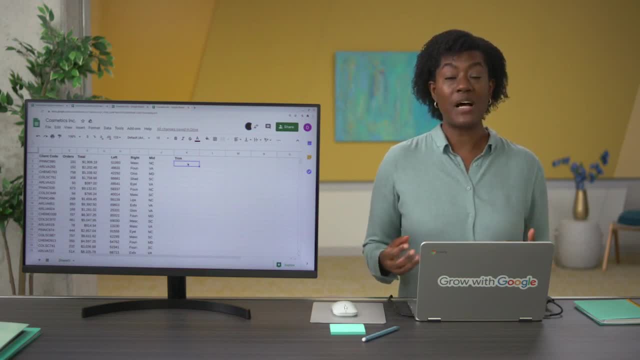 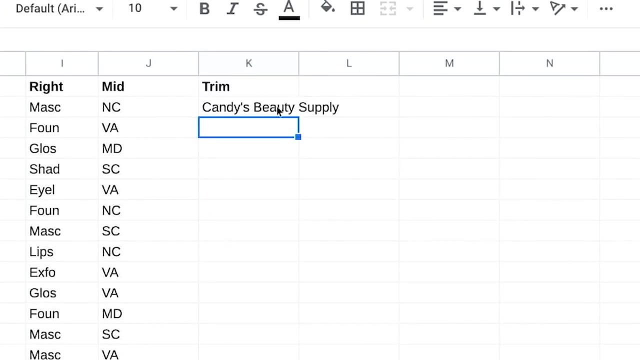 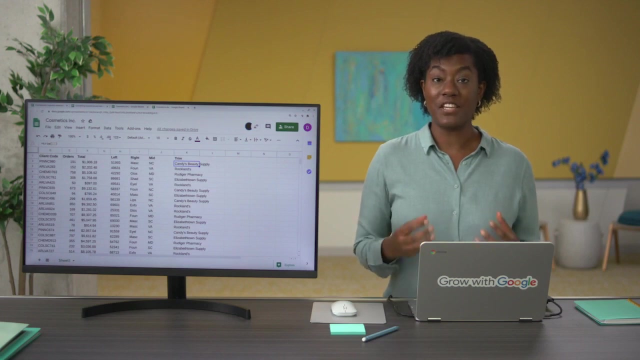 or trailing spaces tag along. These can cause problems when using VLOOKUP, so we want to make sure to use TRIM during the data cleaning process. TRIM automatically deletes any extra spaces added to the cell. Another typical mistake in VLOOKUP which you can easily catch during data cleaning are: 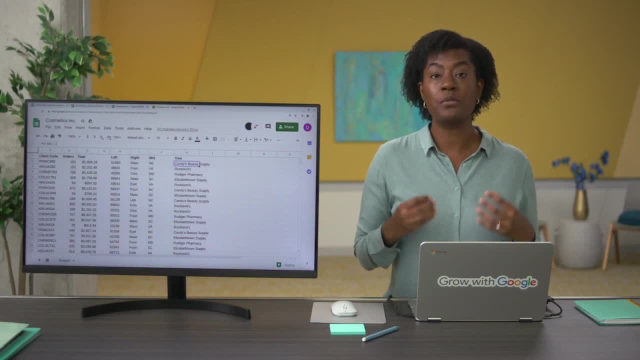 duplicates. If there are duplicate rows in the search, it will return only the first match it finds. As you learned before, remove duplicates is a tool that can be used to find duplicates. If you have duplicate rows in the search, it will return only the first match it finds. 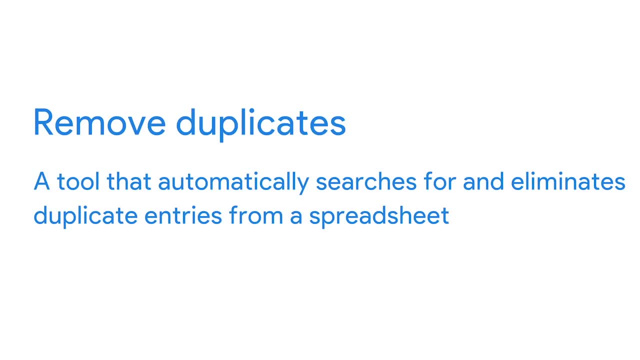 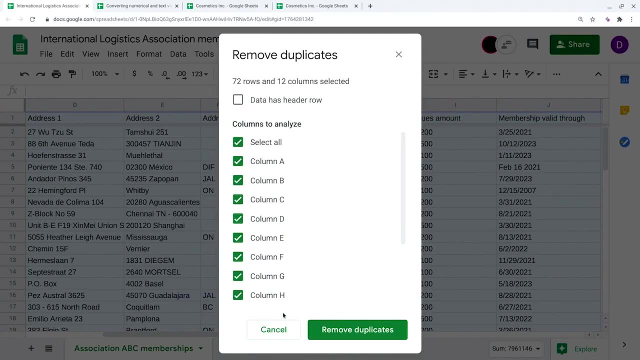 As you learned before, remove duplicates is a tool that automatically searches for and eliminates duplicate entries from a spreadsheet. Using removed duplicates, as you saw in a video a little while ago, is a great way to get rid of duplicates and help make sure you find the right record during the lookup. 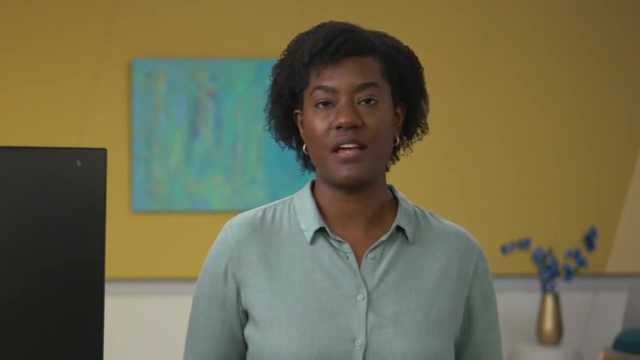 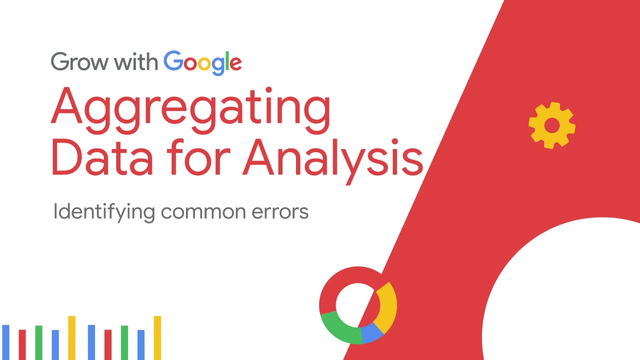 It's always good to remember that clean data is the foundation that everything else is built on, and VLOOKUP can be a very useful data cleaning tool. When people use VLOOKUP, it's important to remember that clean data is the foundation that everything else is built on. 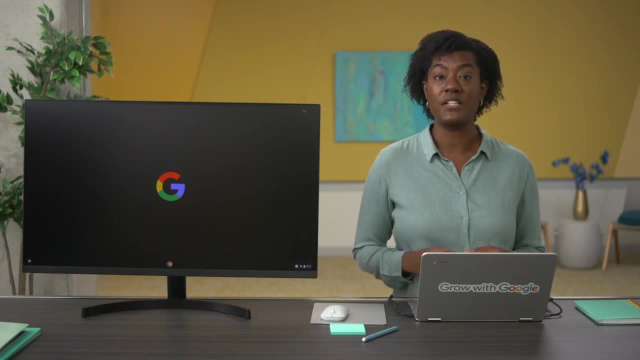 When people start out in data analytics, they often think that those of us who've been in the field for a while know everything. But trust me, we're all still figuring things out, And a lot of the time that means troubleshooting. Troubleshooting has to do with asking the right questions, and that's what we'll focus. 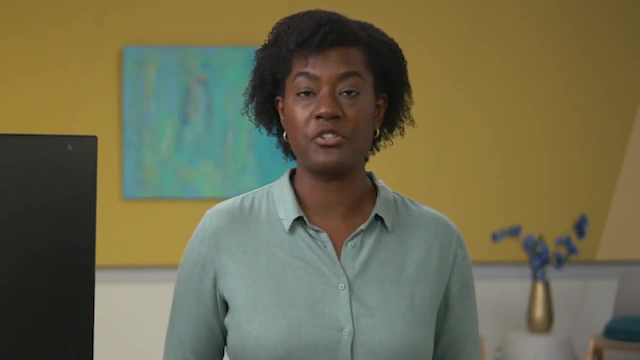 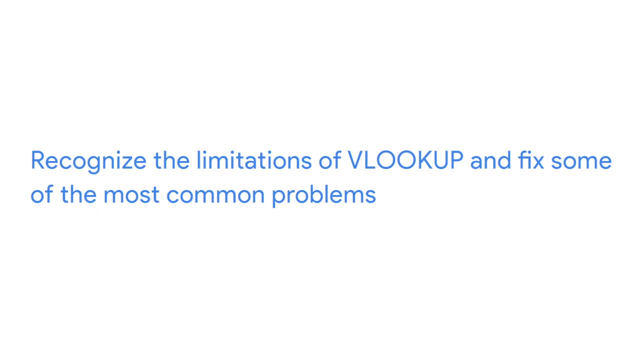 on in this video, We'll learn how you can use troubleshooting to solve all kinds of problems. To do this, we'll need to talk about some of the limitations of VLOOKUP and then practice fixing some of the most common problems that data analysts face. 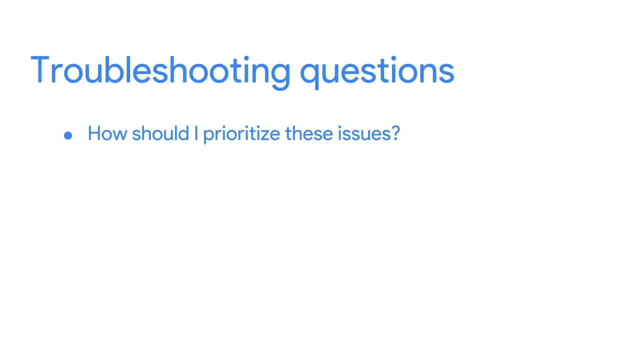 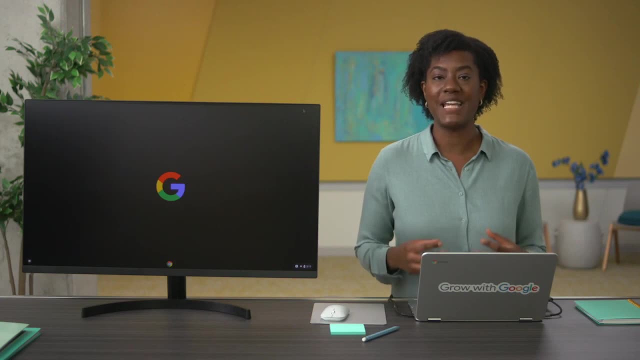 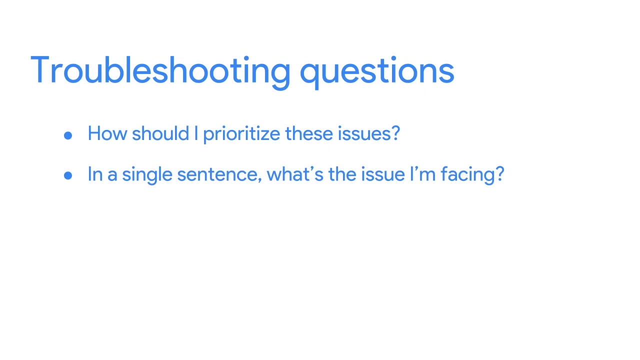 Some of the troubleshooting questions I like to ask myself: How should I prioritize these issues? Trying to solve lots of problems all at once can feel overwhelming. I find it helps when you take things one at a time. Next I ask in a single sentence: what's the issue I'm facing? 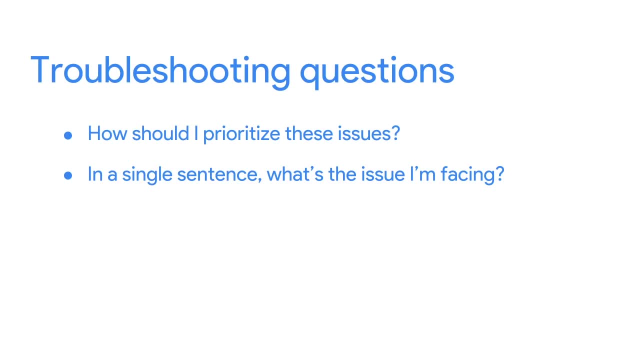 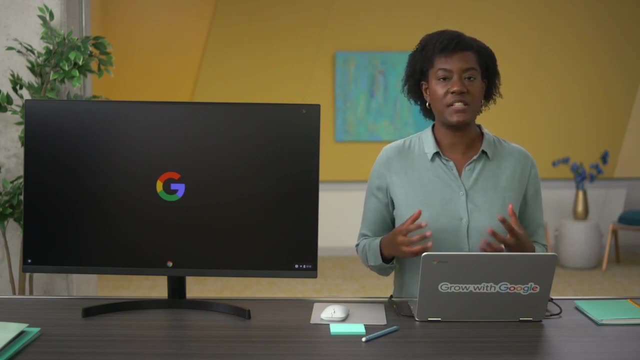 This helps to clarify what's really going on, so I don't get bogged down with extra details. After all, If you don't have a clear objective before looking at the data, you can find just about anything. It's always best to start with your own clear understanding of the situation. 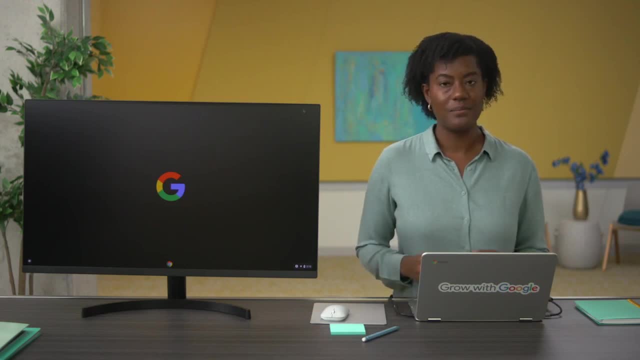 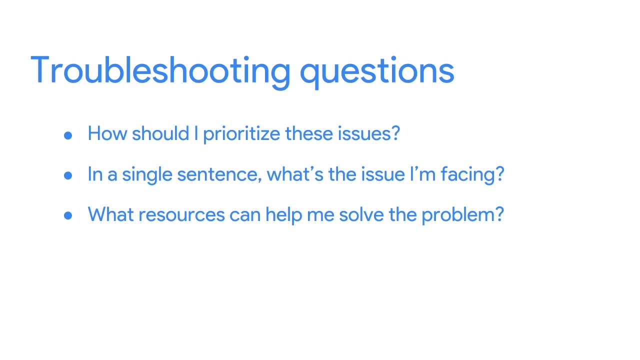 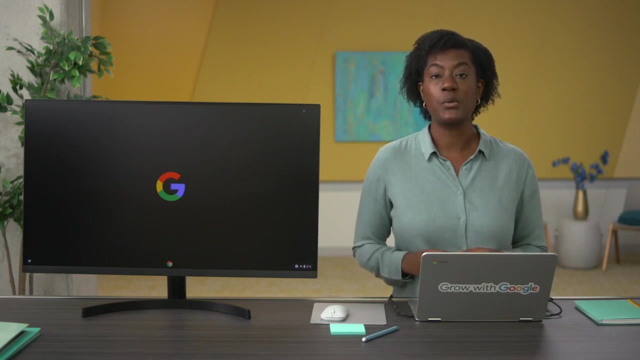 Then let the data tell you if you're on the right track or not. The next question I ask myself is what resources can help me solve the problem. The internet is one of the best resources out there. If you have a question, chances are thousands of others run into exactly the same thing. 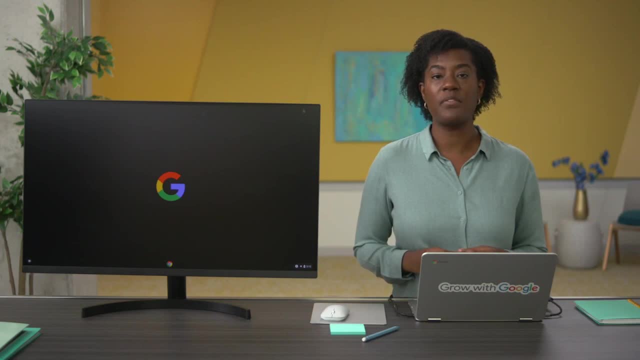 So a quick search can be really helpful, And it's good to remember that people are resources too. Don't be afraid to ask questions. Not only is it a great way to learn, it can also help you build strong relationships with your colleagues. 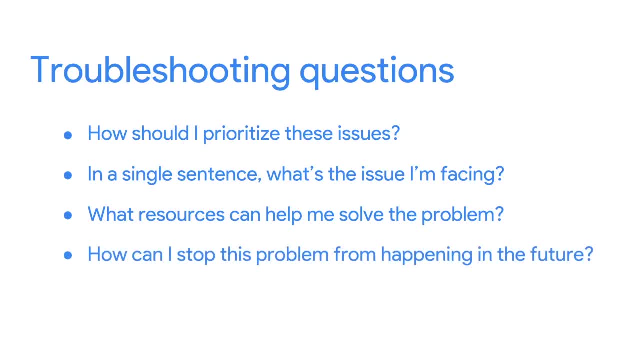 And a final important question I think about: How can I stop this problem from happening in the future. If a new procedure or guideline can stop the same issue from popping up again, that's a great time saver. Alright, Let's start by noting that VLOOKUP only returns the first match it finds. 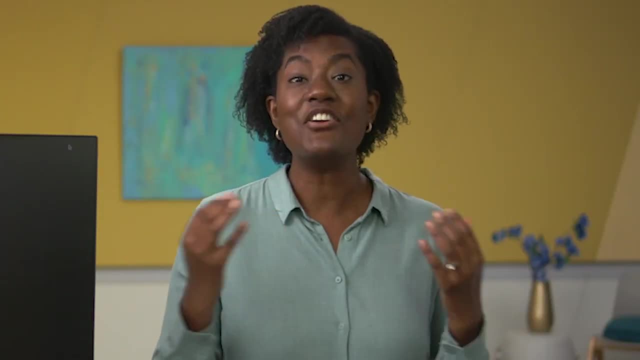 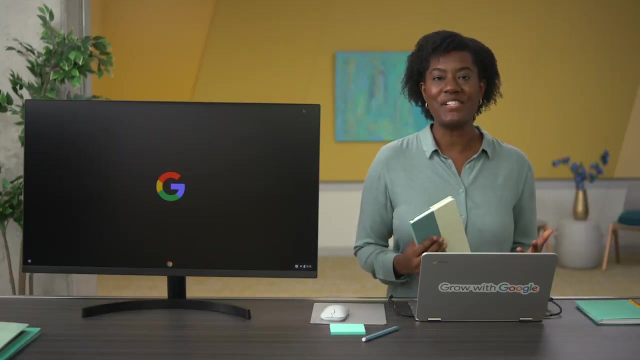 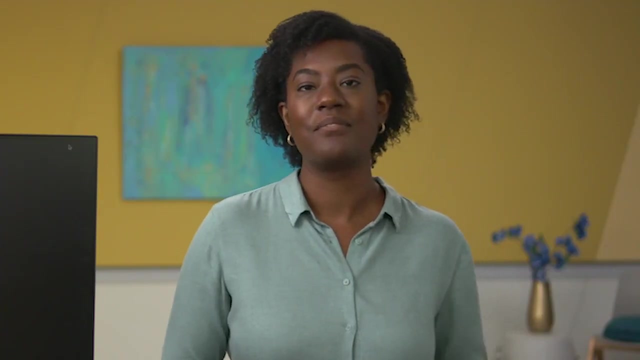 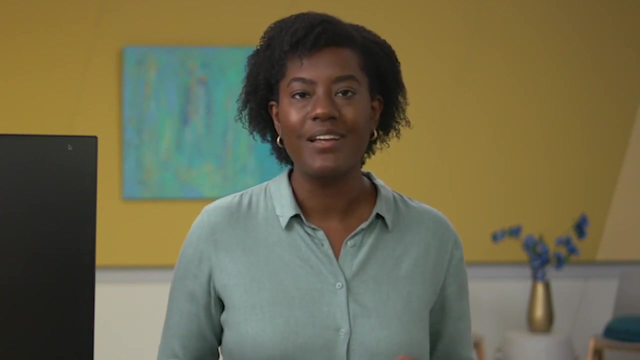 Even if there are lots of possible matches. To understand this, imagine your data set is a phone book. According to research, some of the most popular names are James Smith and Maria Garcia. This means if you need information about the 100th Maria Garcia listed, VLOOKUP won't work. 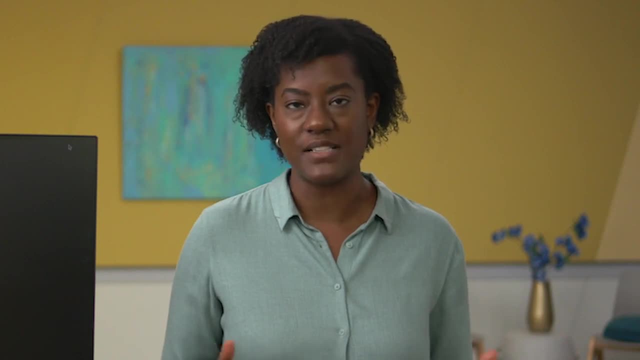 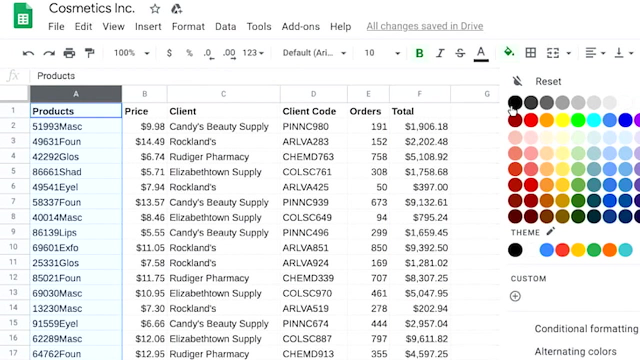 It'll only give you results for the very first Maria it finds. Something else to keep in mind is that VLOOKUP can only return a value from the data to the right. It can't look left. Good news, There's a simple solution. 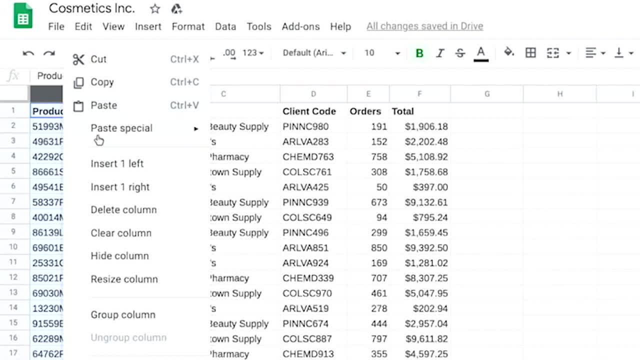 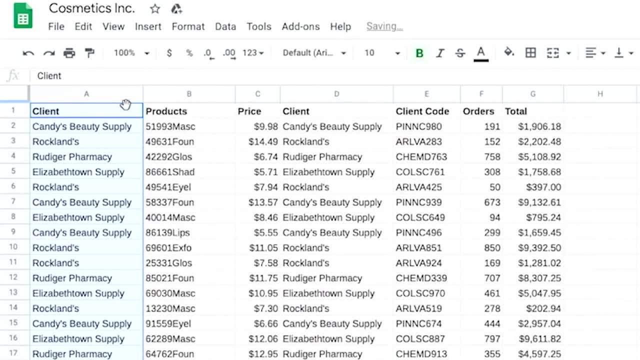 Data analysts usually get around the problem by copying and pasting a column to the left of the data they want to look at This way, the lookup value is in the leftmost column and the data they want is to the right of it. Here's another problem. I see a lot. 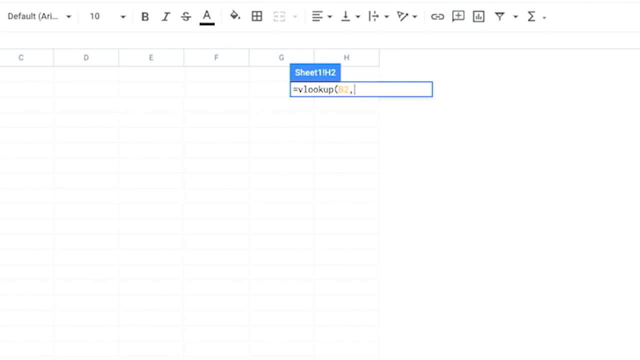 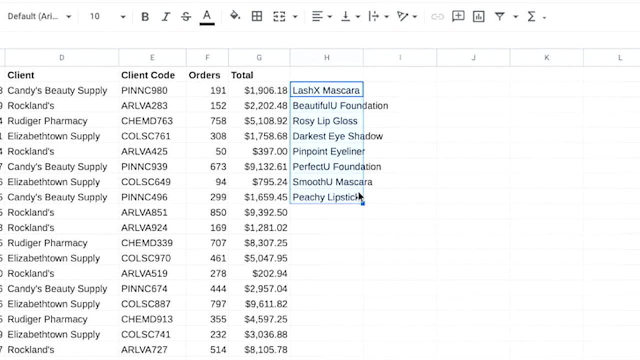 Let's say, the first few rows of a VLOOKUP have returned the correct result, but when you drag the function down the column problems start popping up. This is probably because the table array part of the function hasn't been locked or made absolute. 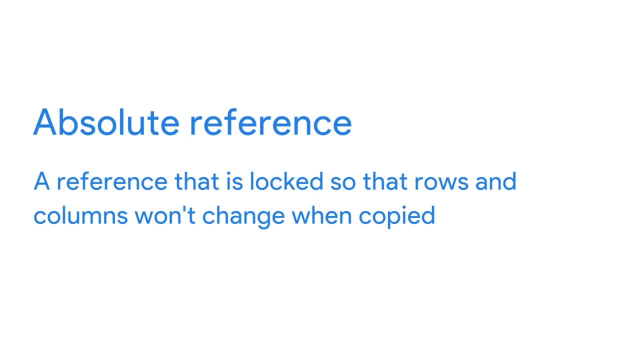 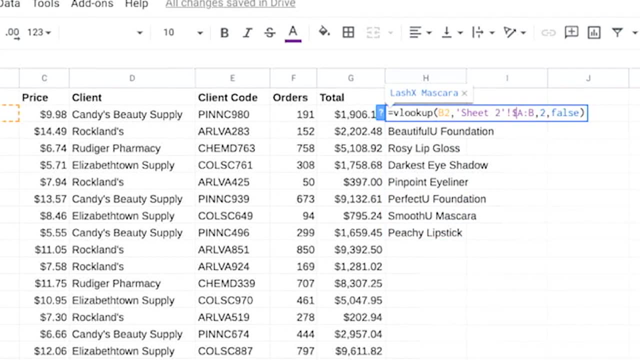 An absolute reference is a reference that is locked so that rows and columns won't change when copied. You can fix this issue by wrapping the table array in dollar signs. As you learned a while back, the dollar sign controls how the reference will be updated. 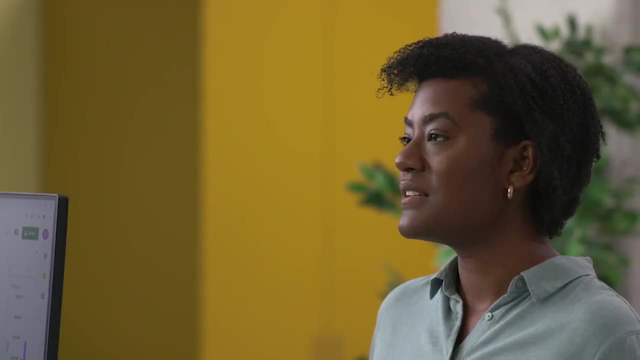 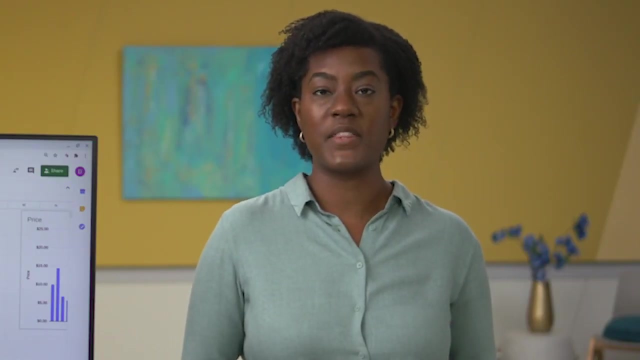 They make sure that the corresponding part of the reference doesn't change Something else that can throw off your VLOOKUP. results are version control issues. In other words, a function worked perfectly at first, but then something in the spreadsheet it was referencing changed. 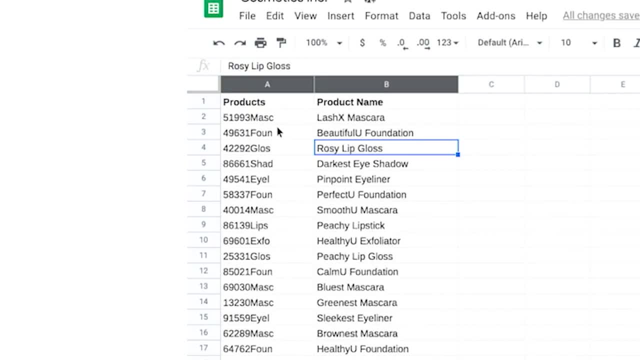 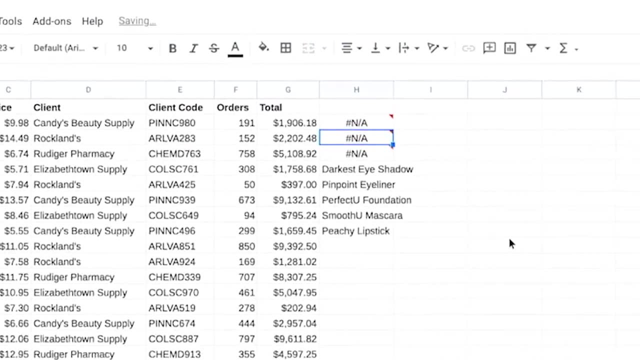 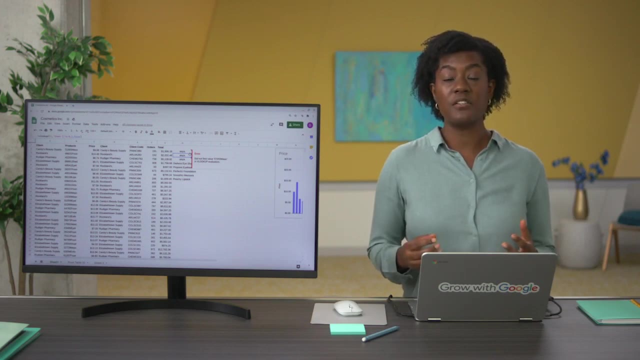 For example, maybe a user inserted a column, So now the columns in your function no longer direct VLOOKUP to the right place. When something like this happens, it'll return an incorrect value. There are a few actions data analysts can take to ensure this doesn't happen. 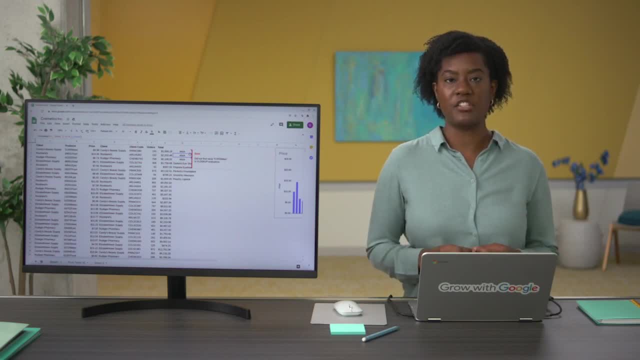 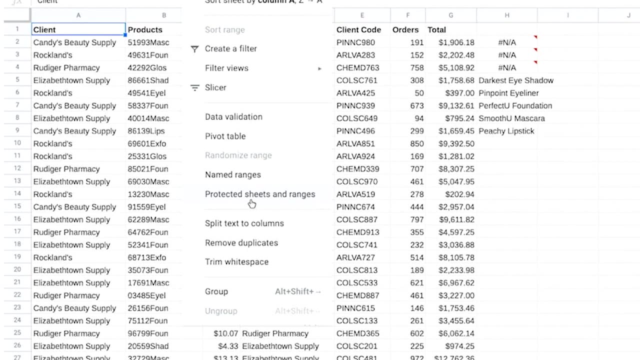 First lock the spreadsheet. This stops other people from making changes To do this in Sheets. select Data, then Protected Sheets and Ranges In other spreadsheet applications. there are other tools that do the same thing. Next, choose what you want to protect. 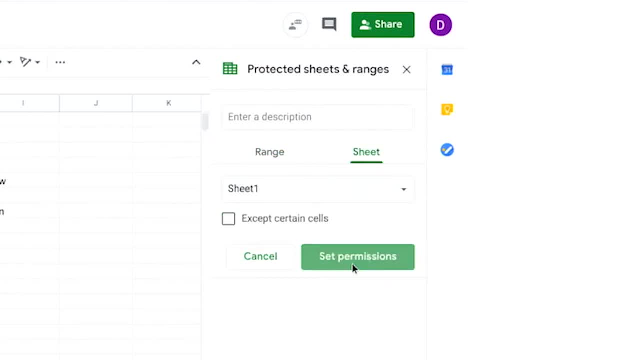 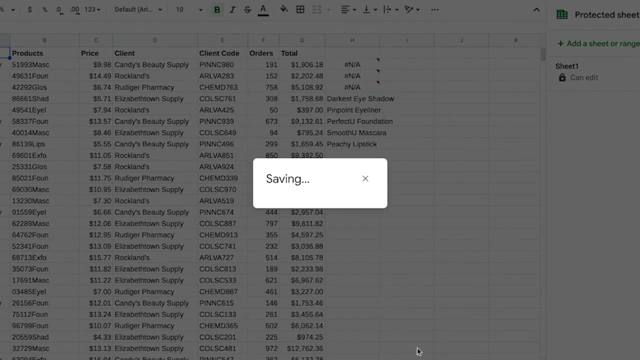 In this case, we want to protect the entire sheet. Then you can set permissions to either show a warning or restrict who can edit. Choose only you, then done. But keep in mind there will be times when other people need to be protected. 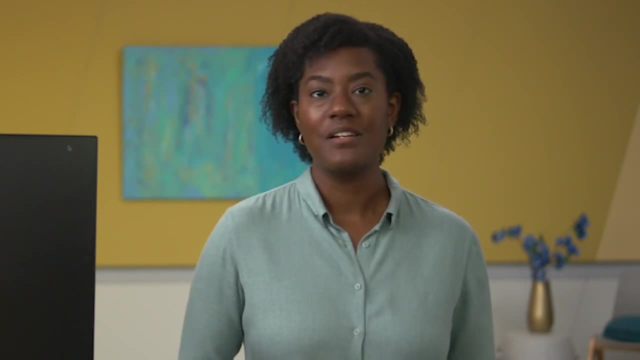 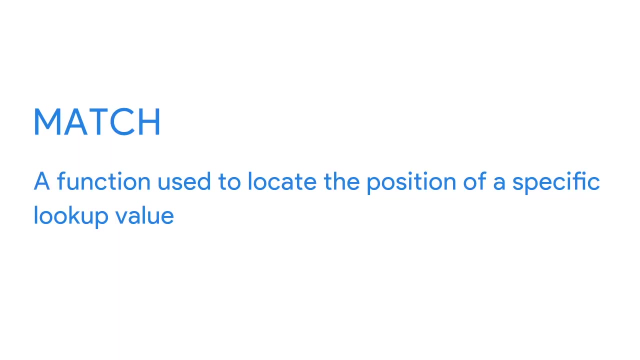 This is because the data is protected. This is because the data is protected, So locking them out might make you pretty unpopular with your coworkers. When that's the case, you can use MATCH, which is a function used to locate the position of a specific lookup value and can help you with version control. 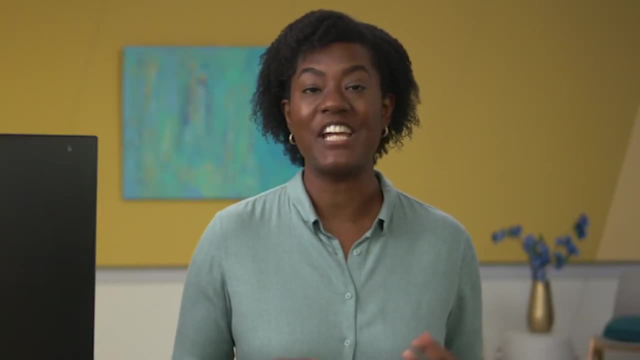 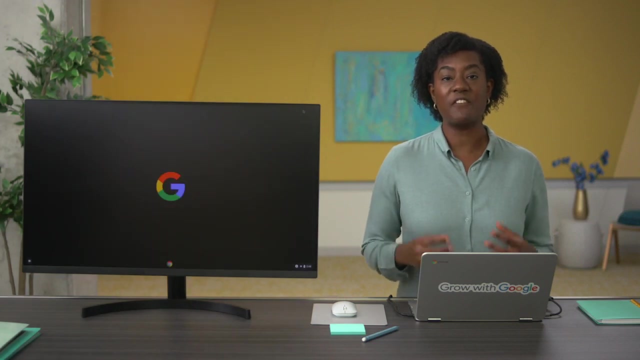 We won't get into that right now, but just know that it's an option in case you ever need it. The final problem we'll talk about has to do with exact and approximate matching. When using VLOOKUP, you're likely to get different results depending on whether you enter the 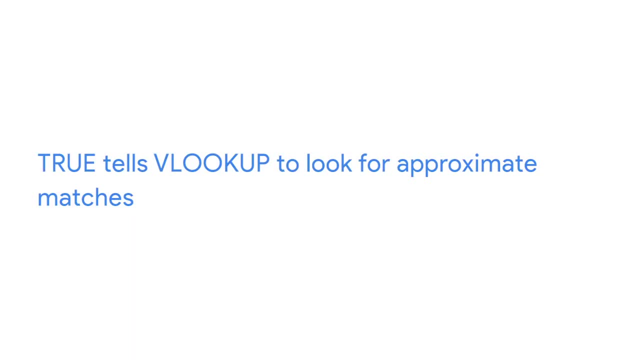 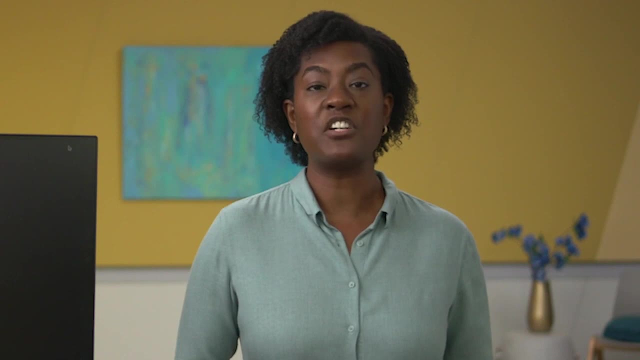 word TRUE or FALSE within your function. TRUE tells VLOOKUP to look for approximate matches and FALSE tells VLOOKUP to look for exact matches. So if a function looks like this, it's telling VLOOKUP to find the closest match to the text. 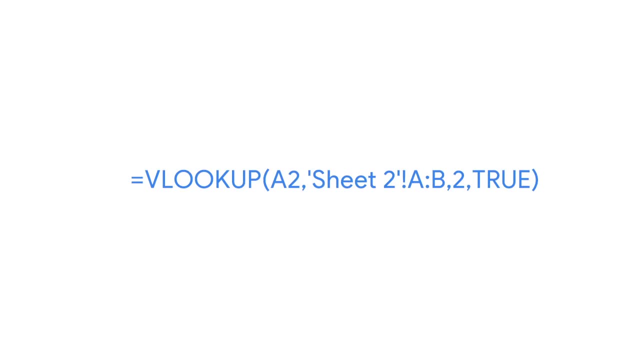 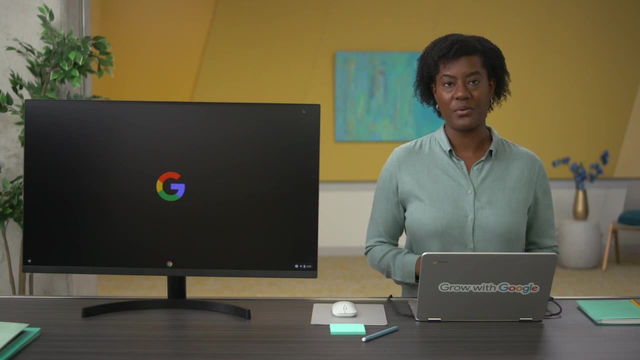 or number we're looking for. It's important to note that VLOOKUP starts at the top of a specified range and searches downward vertically in each cell to find the right value. It stops searching when it finds any value that's greater than or equal to the value. 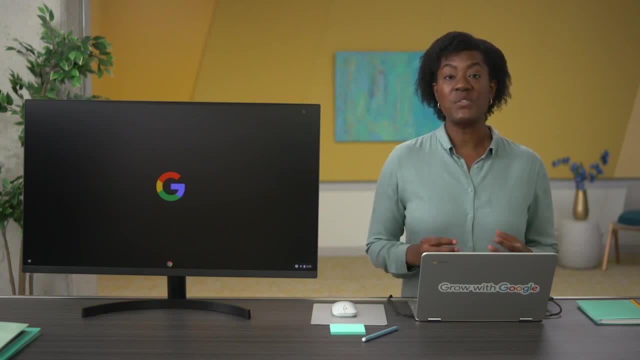 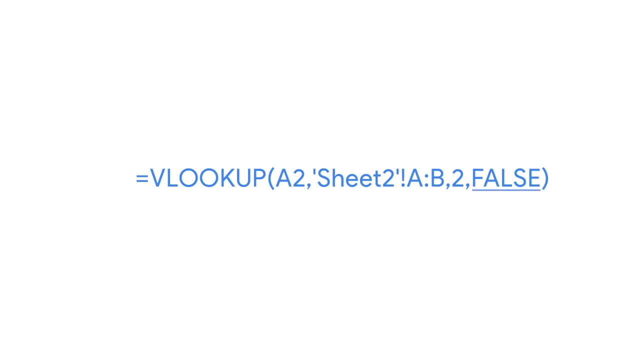 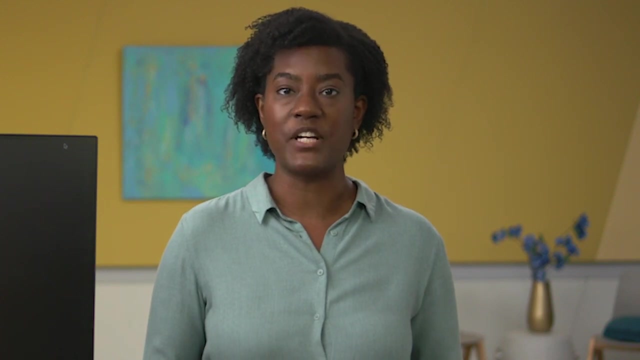 we're looking for. That's why data analysts typically use FALSE like this. That way, VLOOKUP only returns the exact match to what you've entered in the lookup value. VLOOKUP is one of the most popular lookup and reference functions in spreadsheets. 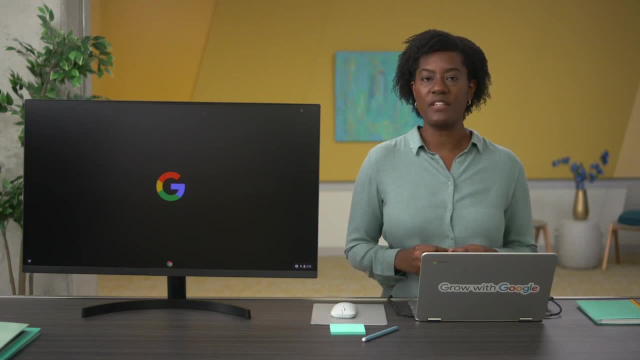 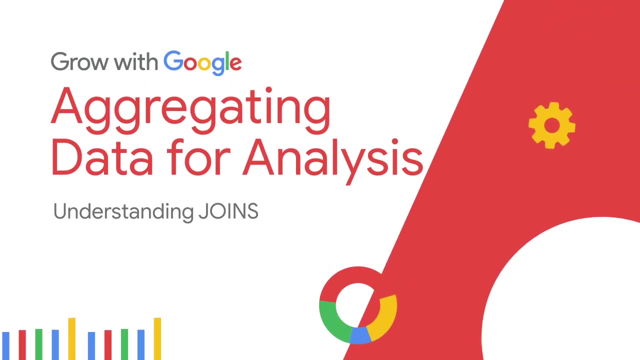 It's also one of the trickiest Coming up. you'll learn about more of these common challenges. Everything you learn will help you run into fewer problems when you start using VLOOKUP as a future data analyst. So far, we've checked out a few different tools you can use to aggregate data within. 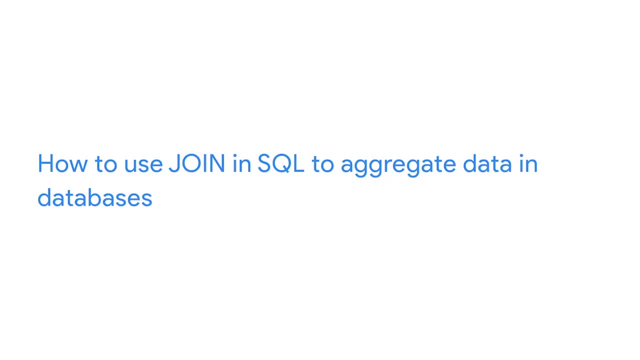 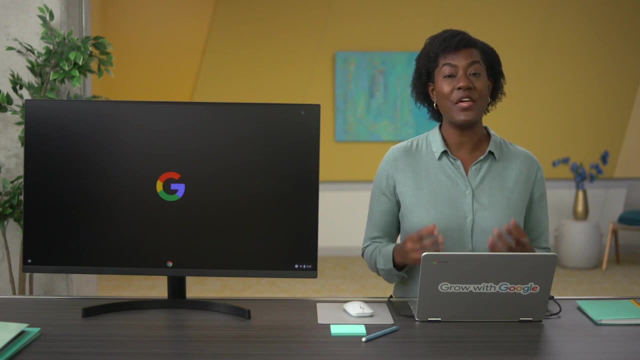 spreadsheets. In this video we'll cover how to use JOIN and SQL to aggregate data in databases. First I'll tell you a little bit about what a JOIN actually is, and then we'll explore some of the most common JOINs in action. 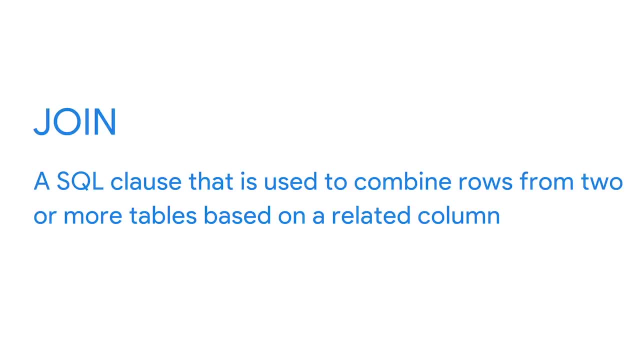 Let's get started. JOIN is a SQL clause that's used to combine rows from two or more tables based on a related column. Basically, you can think of JOIN as the SQL version of VLOOKUP, which we just covered. There's four common JOINs data analysts use – INNER, LEFT, RIGHT and OUTER. 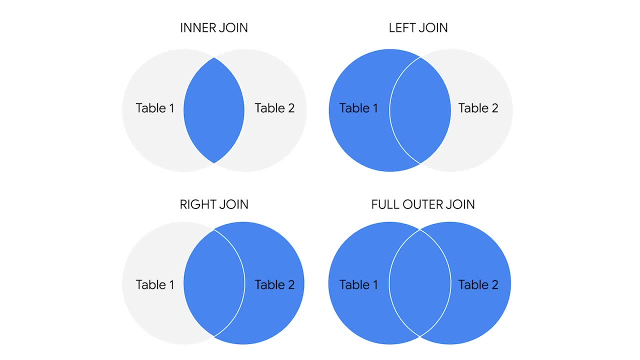 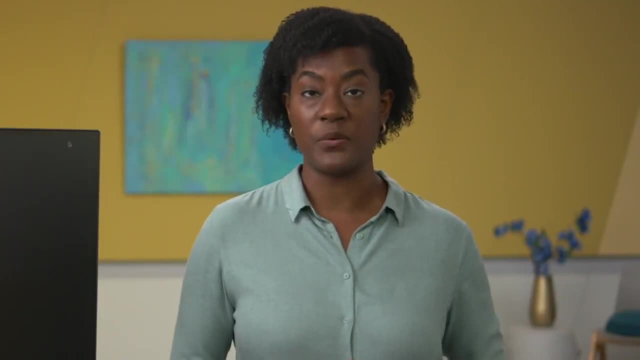 Here's a handy visualization of what each JOIN actually does. We'll use these to help us understand these functions. JOINs help you combine matching or related columns from different tables. When we learned about relational databases, we referred to them in our previous video. 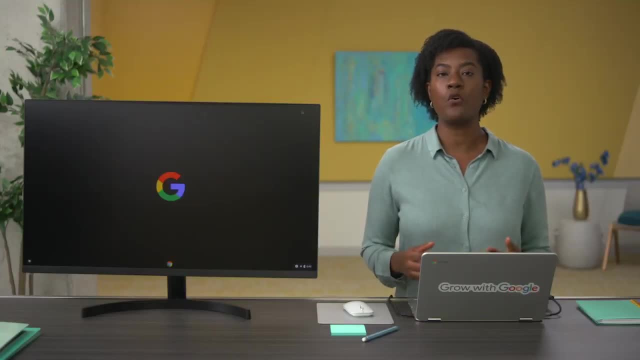 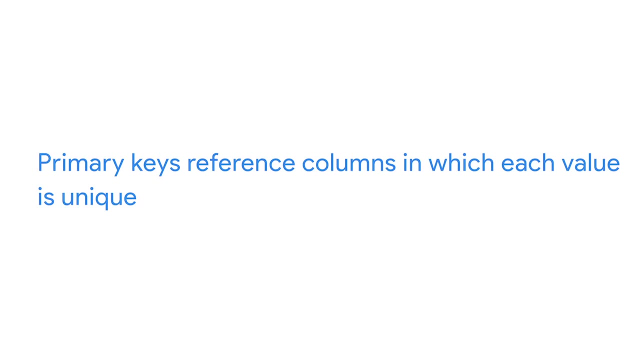 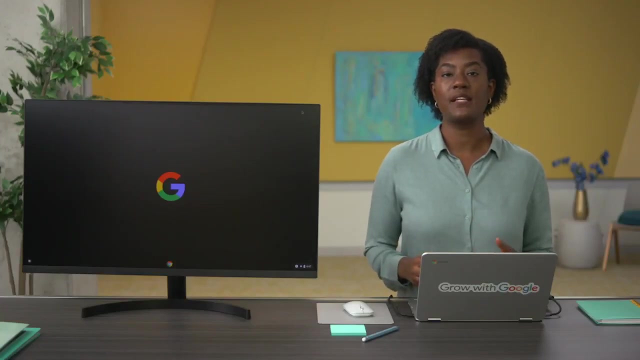 So let's get started. JOIN refers to these values as primary and foreign keys. Primary keys: reference columns in which each value is unique to that table. But that table can have multiple foreign keys which are primary keys in other tables. For example, in a table about employees, the employee ID is the primary key and the office. 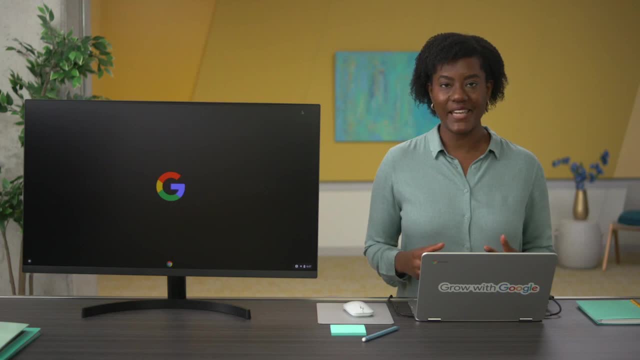 ID is a foreign key. JOINs use these keys to identify relationships and corresponding values. An INNER JOIN is a function that returns records from the table. We'll be using the INNER JOIN function to identify relationships and corresponding values. An INNER JOIN is a function that returns records for the same table. 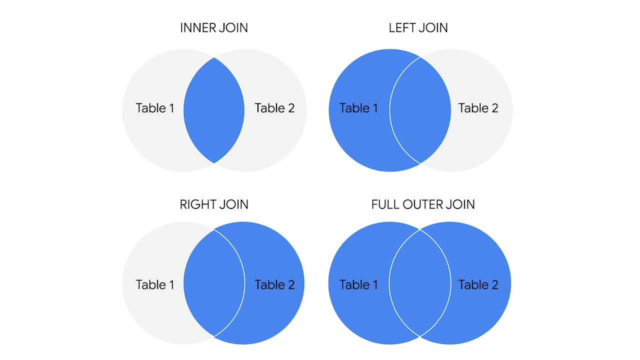 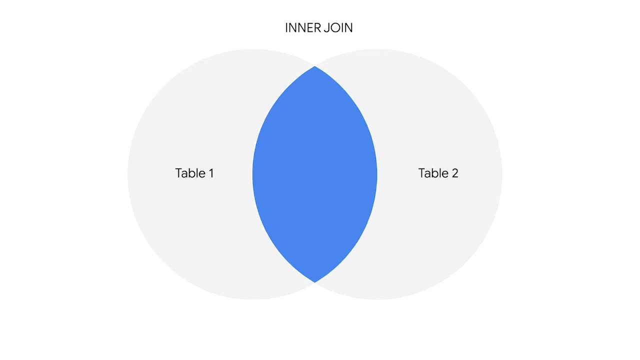 records with matching values in both tables. If we think about our tables as the circles of this Venn diagram, then an inner join would return the records that exist where the tables are overlapping. For the records to appear in the results table, there has to be key values in both tables. 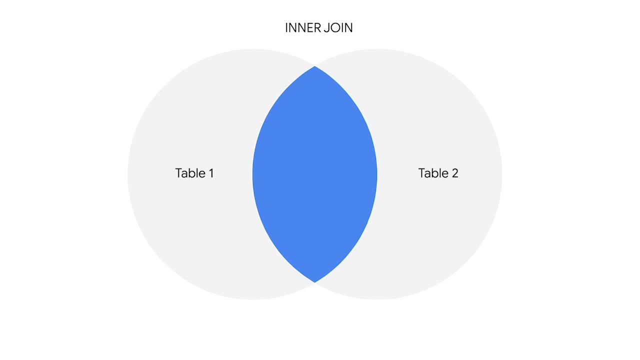 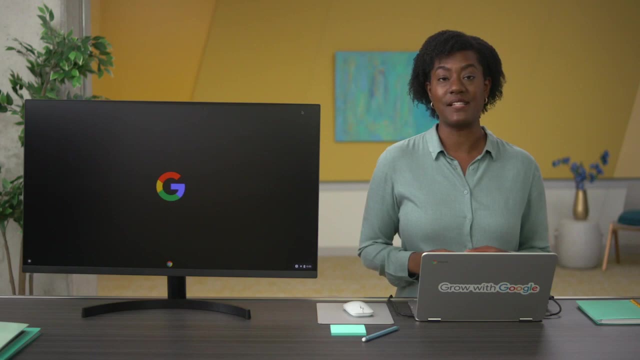 The records will only merge if there's matches in both tables. When you input join into SQL, it usually defaults to inner join, so a lot of analysts will use join as shorthand instead of typing the whole query. A left join is a function that will return all the records from the left. 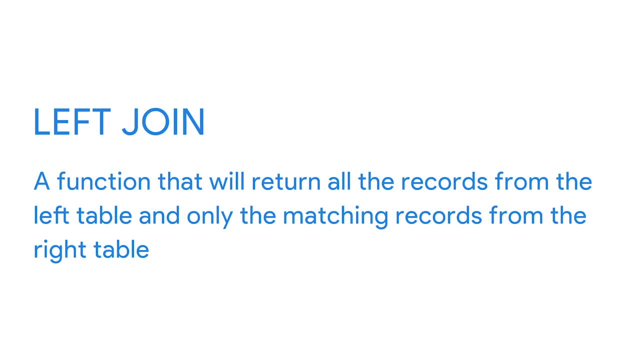 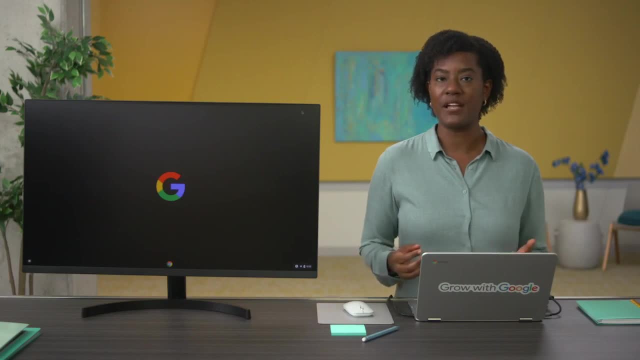 table and only the matching records from the right table. Here's how you can figure out which table is left or right. In English and SQL we read from left to right. so the table mentioned first is left and the table mentioned second is right. You can also think of left as the table name to the left. 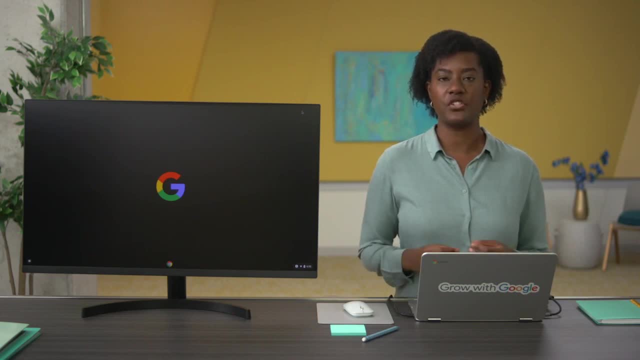 of the join statement and right as the table name to the right of the join statement. In this diagram, we can see that the table name to the left of the join statement is left and the table to the right of the join statement is right. In this diagram, you'll notice that the entire left. 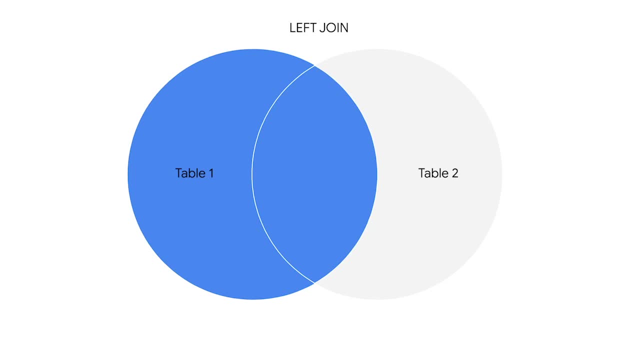 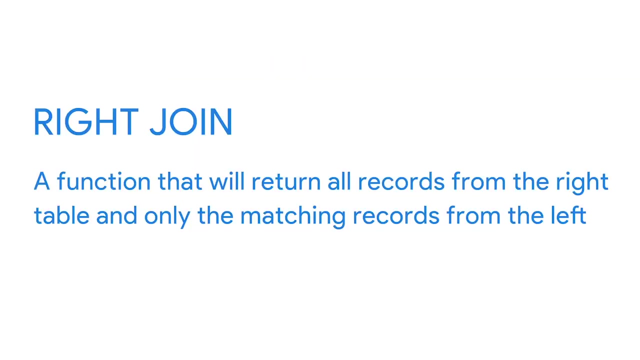 table is colored in and the overlap with the right table, which shows us that the left table and the records it shares with the right table are being selected. Each row in the left table appears in the results, even if there's matches in the right table. Right join does the opposite. It will return. 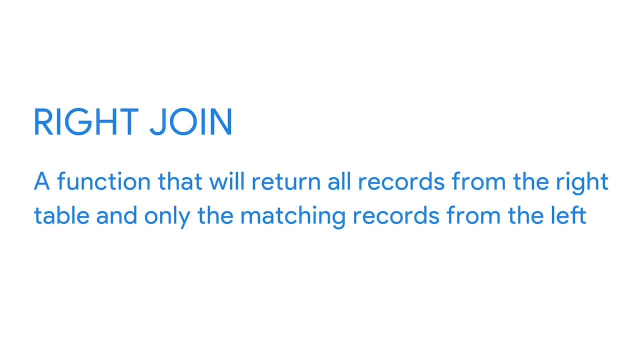 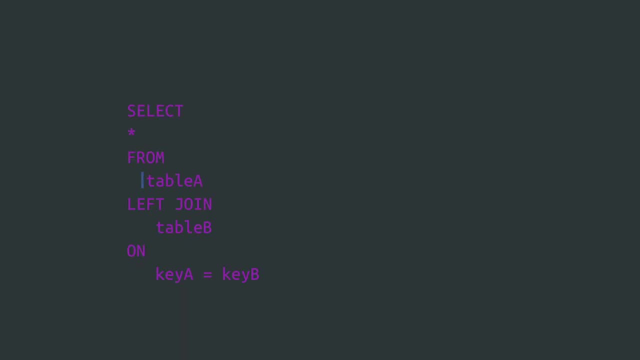 all records from the right table and only the matching records from the left. You can get the same results if you flip the order of the tables and use a left join. For example, select from table A- left join table B is the same as select from table B- right join table A. 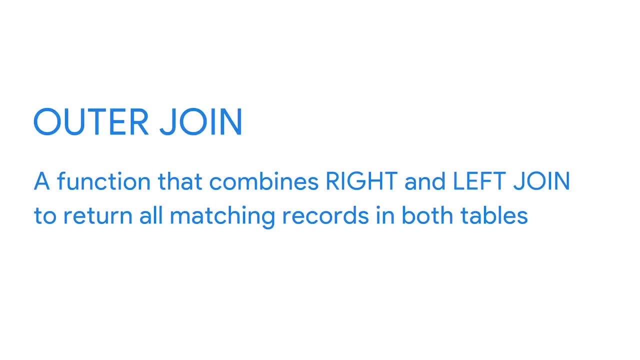 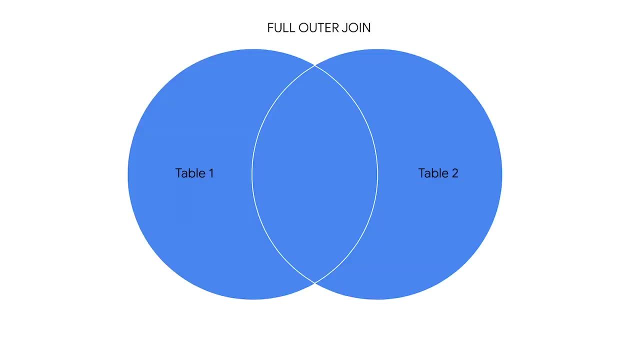 Finally, there's outer join. Outer join combines right and left join to return all matching records in both tables. This means it'll return all records in both tables. If there's records in one table without a match, it'll create a record with null values for the other table, Using joins. 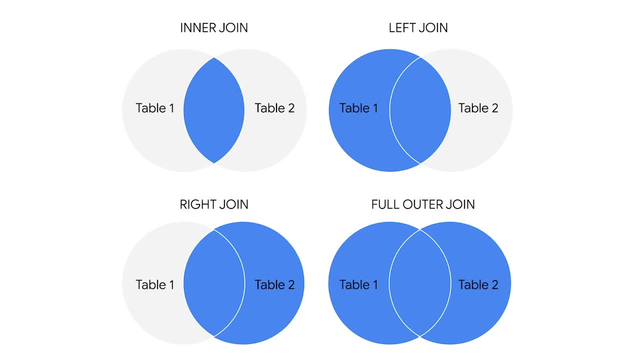 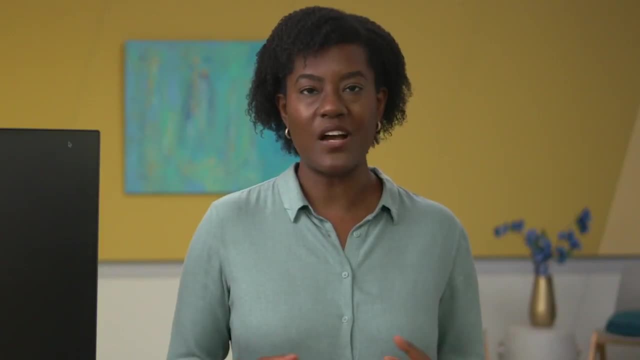 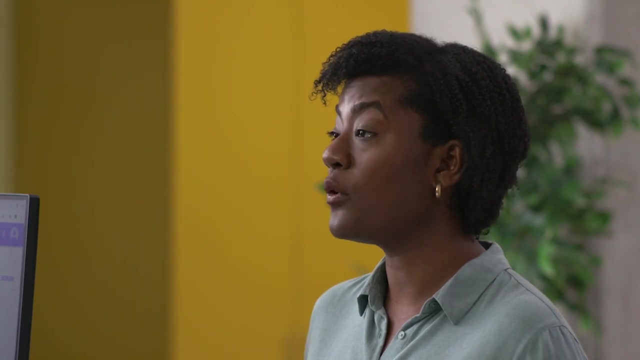 can make working with multiple data sources a lot easier and it can make relationships between tables more clear, But unfortunately they don't work in SQL. Let's find out why. Here's an example. Let's say you're working with employee data across multiple departments. We have an employee's table. 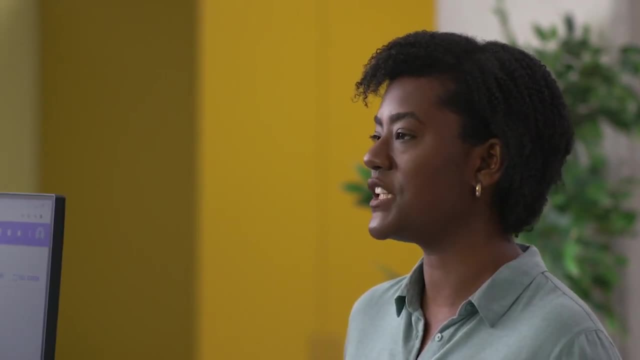 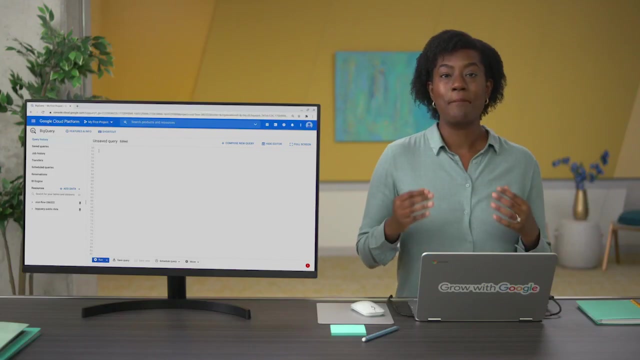 and a department's table which both have some columns like department ID. We can use different join clauses to help us pull different data from our tables and aggregate it. Maybe we want to get a list of employees with their department name, excluding any employee without a department ID. 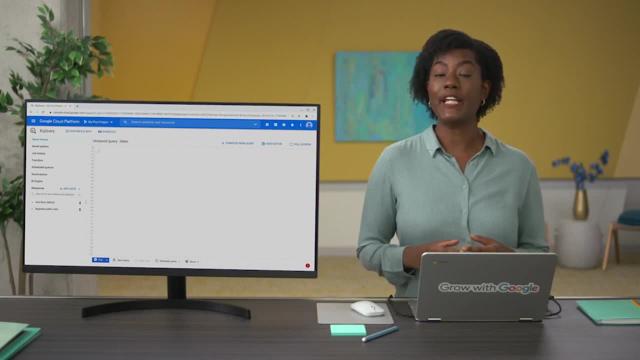 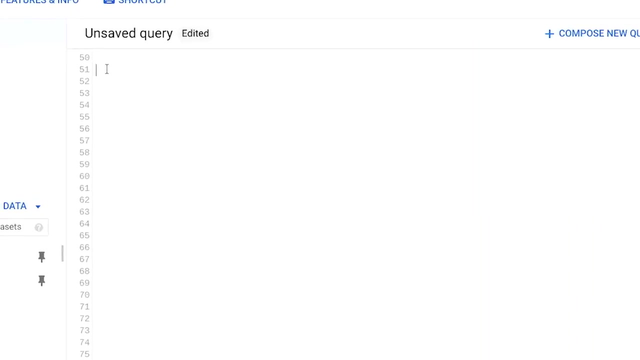 Because a department ID record is used in both tables, we can use an inner join to return a list with only those employees. As a quick reminder, analysts will sometimes just input join for an inner join, but for this example we'll write it out. So to build this query, 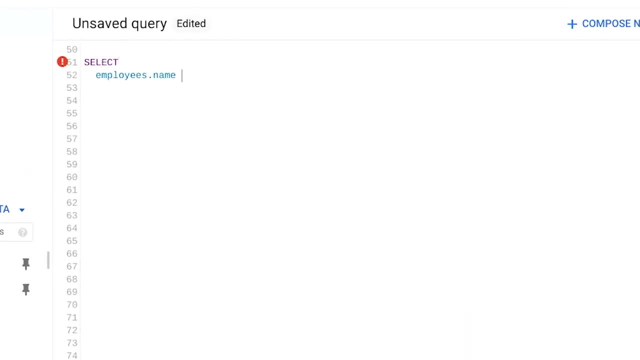 we'll start with select and as to tell SQL how we want the columns titled. Then we'll use from to tell it where we're getting this data, in this case the employees table, And then we'll input inner join in the other table we're using, which is departments. 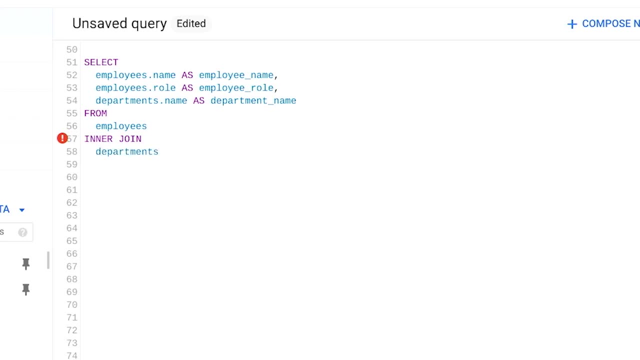 We can specify which column in each table will contain the matching join key by writing on employees dot. department underscore ID equals department ID. We can also specify the ID for each column in the table: departmentsDepartments underscore ID. Now let's run it. 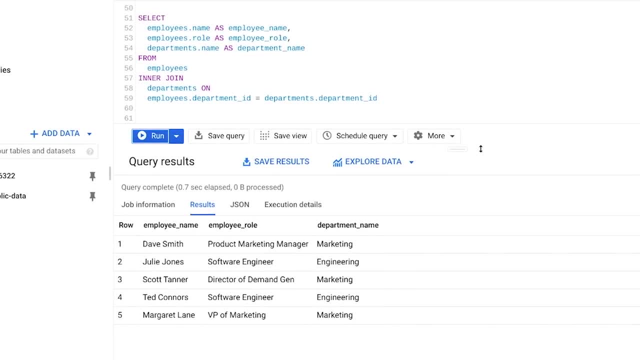 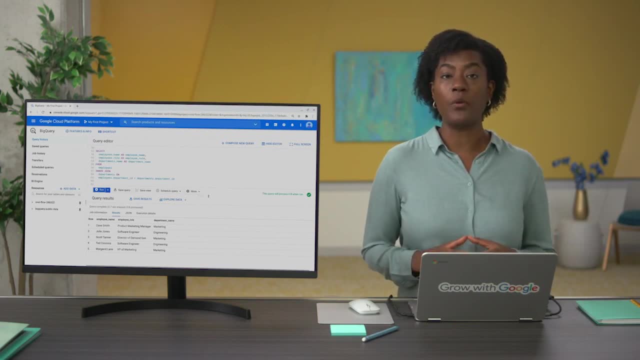 And there Now we've got a list of employee names and department IDs for the employees that have those IDs, But we could use left or right join to return a list of all employee names and their departments when available. Let's try both really quickly. 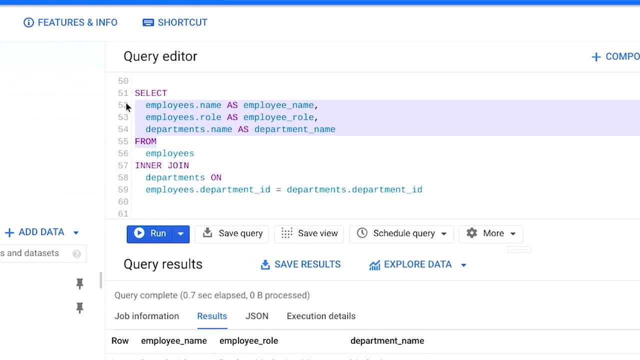 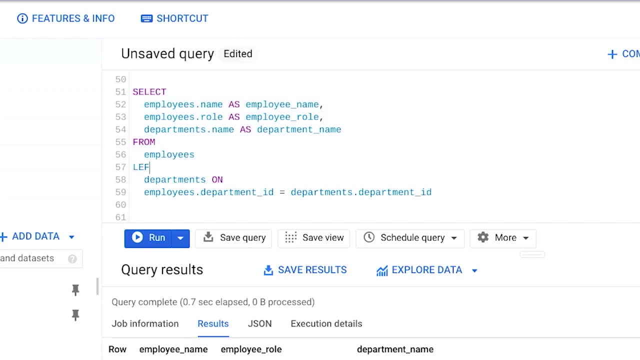 So this will start similar to the last query. We'll put in select as and from again, But this time we'll say left, join and use on, like we did with the last query. When we execute the query, we get back this new list. 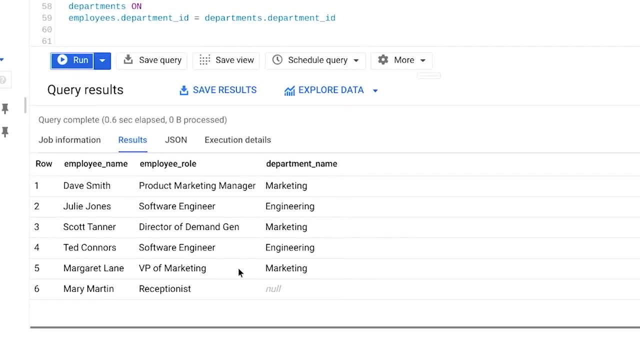 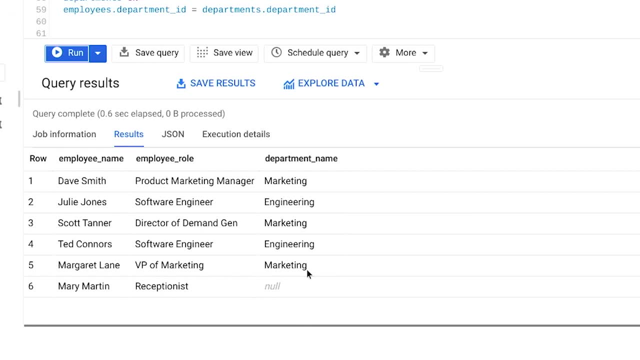 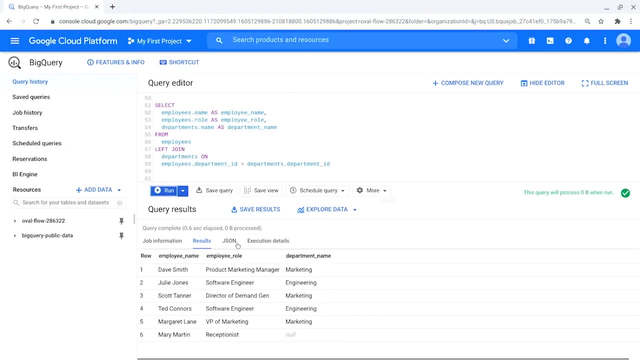 with the employee names and departments, But you'll notice there's null values. These are places where the right table, which is departments in this case, didn't have corresponding values. Let's try right join, just to test it out. This query will be almost the same. 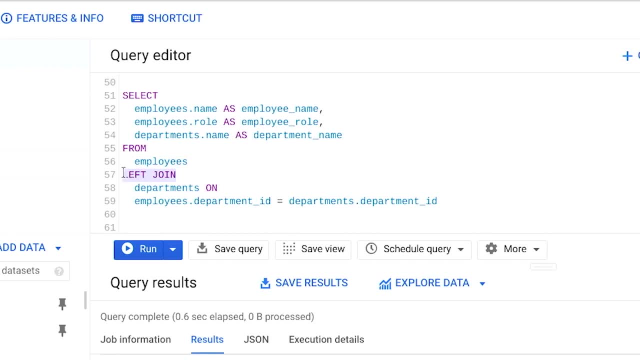 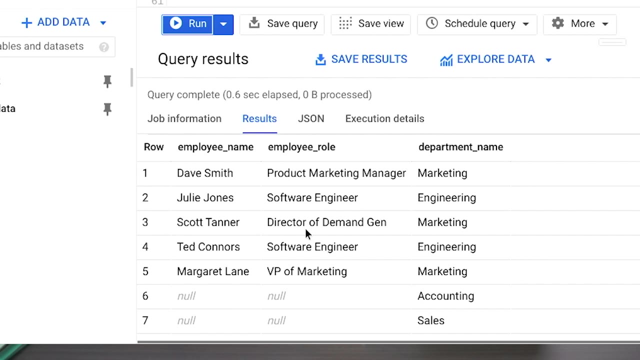 Only difference is that we'll use the right join clause to return all of the rows from the right table, whether they have matching values in the table to the left of the join statement or not. In this case, the right table is employees. Now let's try out one last join outer. 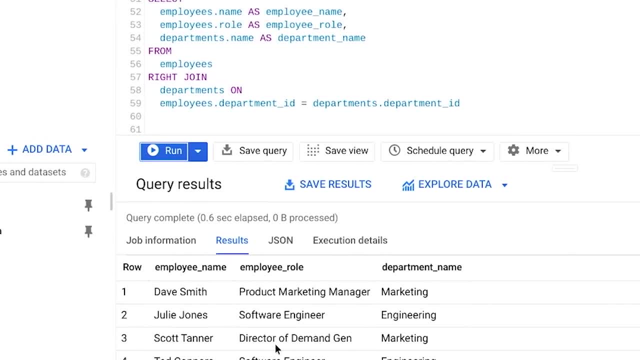 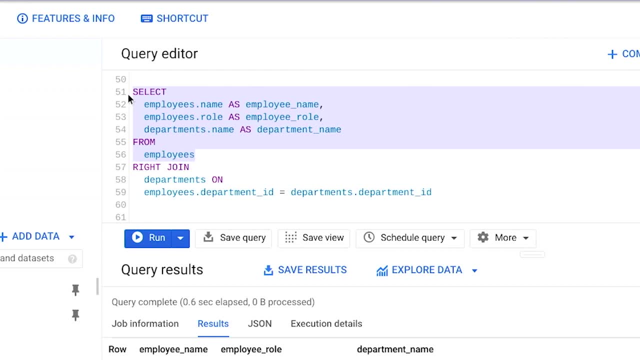 Outer join will fetch all of the employee names and departments. This query will start a lot like the other ones we've done. We'll use select as and from to choose what data we want and how. We'll grab this from the employees table and put full outer join with the departments table. 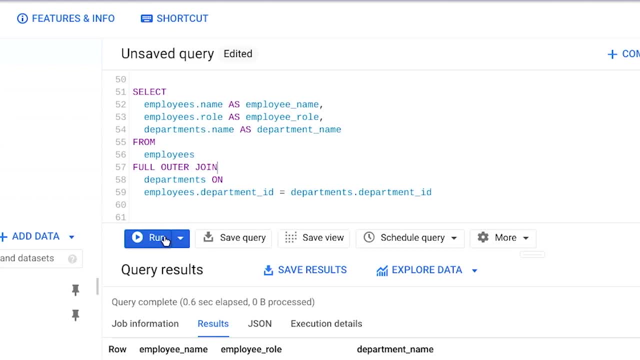 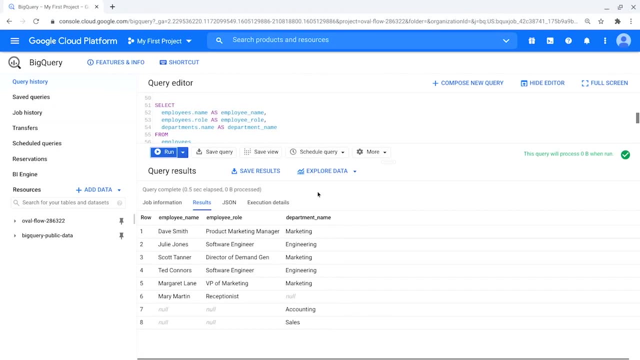 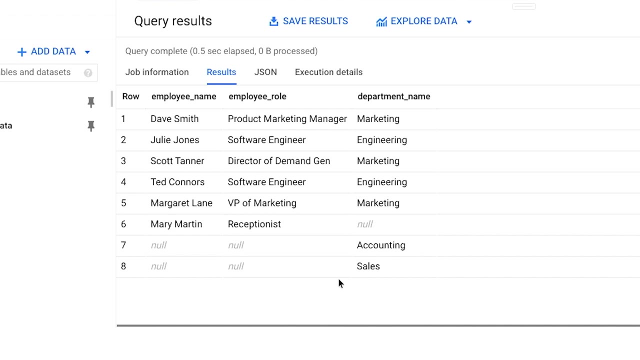 to get all of the records from both. We'll also use on again here. Now we can run this And we'll get all of the employee names and departments from these tables. There will be nulls because we've joined columns that don't have matching values. 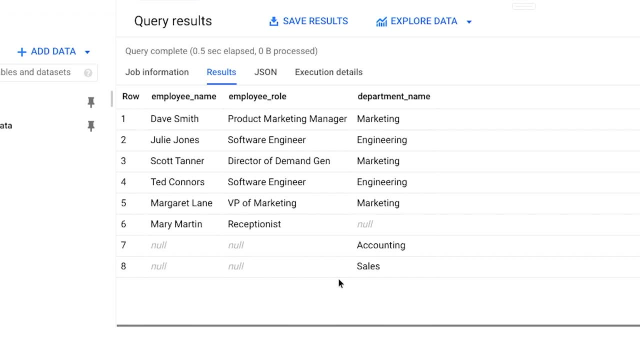 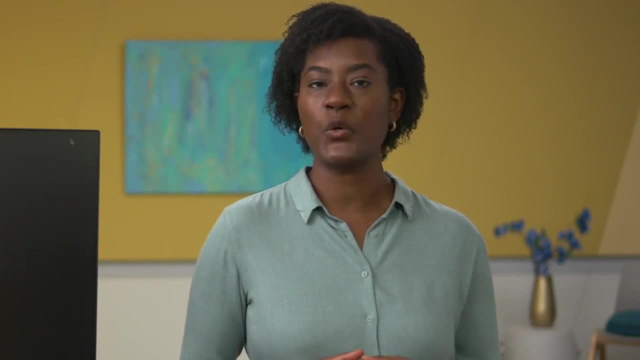 And there Now you know how joins work. Joins are super useful when you need to work with data from multiple related tables. They give you a lot of flexibility with how you combine and view that data And if you ever have trouble remembering what inner, right, left or outer join do. 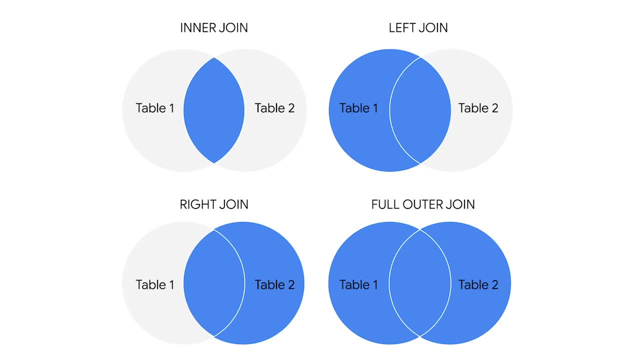 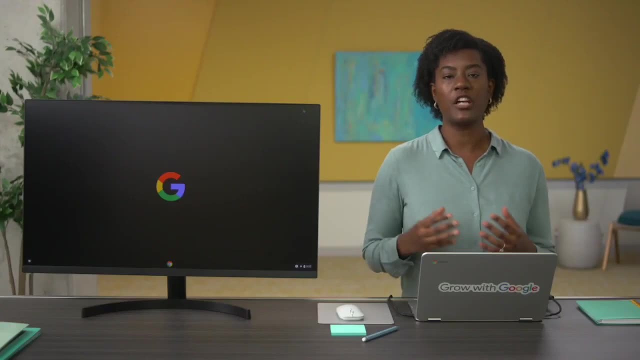 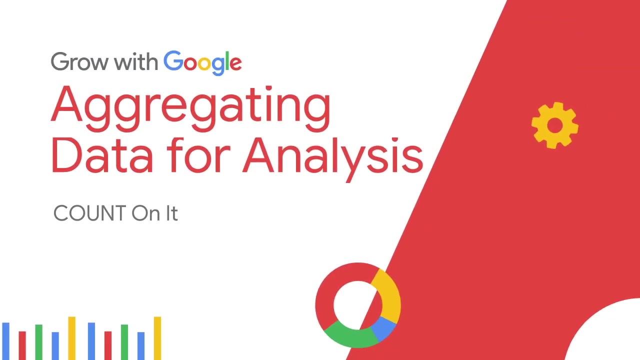 just think back to our Venn diagram. We'll keep learning about aggregating data in SQL in the next video. Thank you, We'll see you in SQL next time. See you soon. By now we've discovered that spreadsheets in SQL. 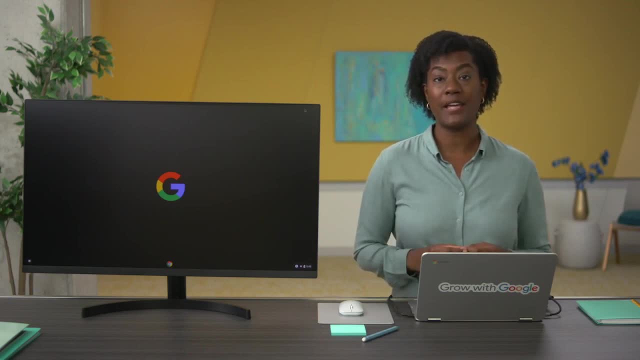 have a lot of tools in common. Earlier in this program we learned about count in spreadsheets. Now it's time to look at similar tools in SQL: count and count distinct. In this video we'll talk about when you'd use these queries. 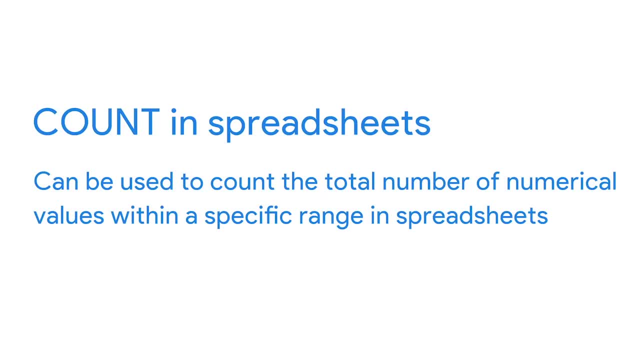 and check out an example. Let's get started. Count can be used to count the total number of numerical values within a specific range in spreadsheets. Count in SQL does the same thing. Count is a query that returns the number of rows in a specified range. 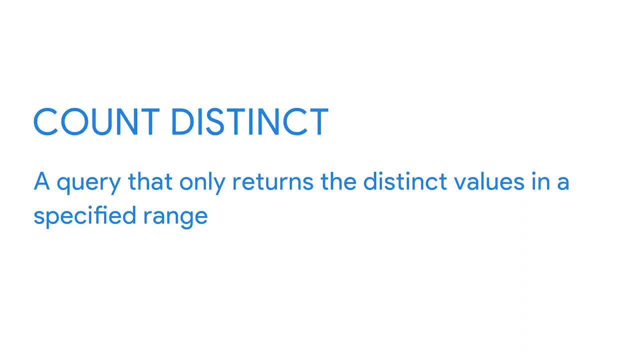 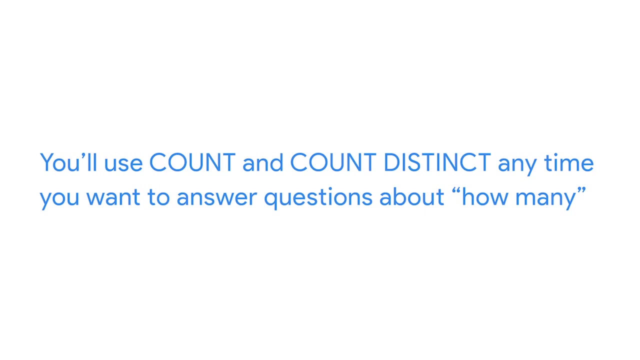 But count distinct is a little different. Count distinct is a query that only returns the distinct values in that range. Basically, this means count distinct doesn't count repeating values. As a data analyst, you'll use count and count distinct any time you want to answer questions about. 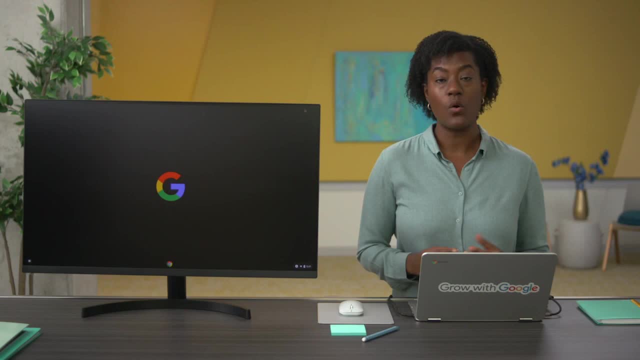 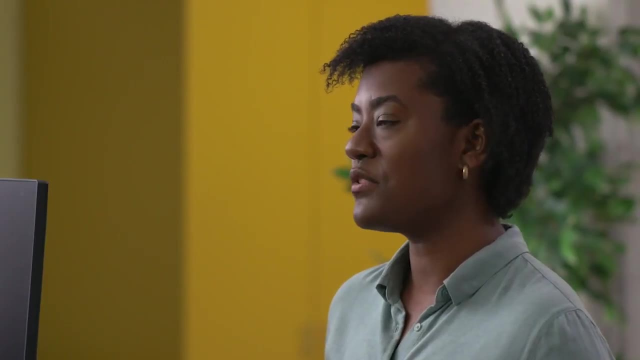 how many Like, how many customers did this or how many transactions were there this month or how many dates are in this data set, And you'll use them throughout the data analysis process at different stages. For example, you might need them while you're cleaning data. 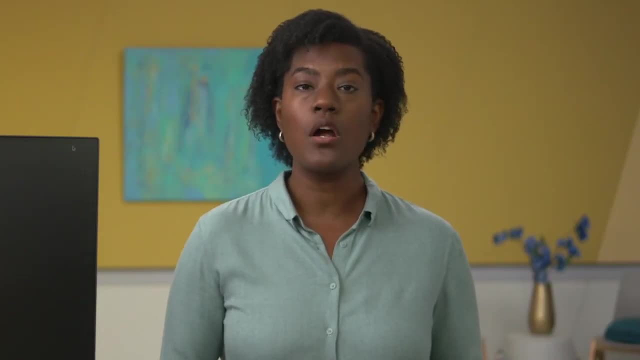 to check how many rows are left in your data set. Or you might use count and count distinct during the actual analysis to answer a how many question. You'll run into these kinds of questions a lot, So count and count distinct are really useful to know. 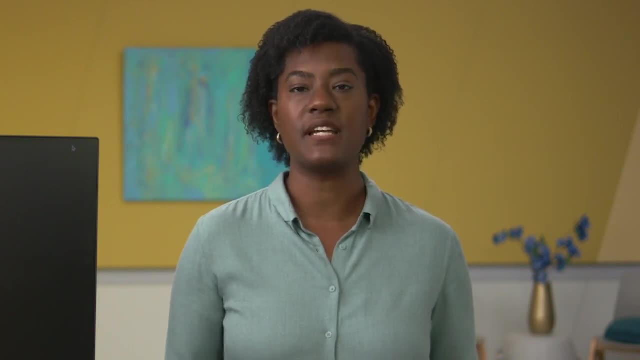 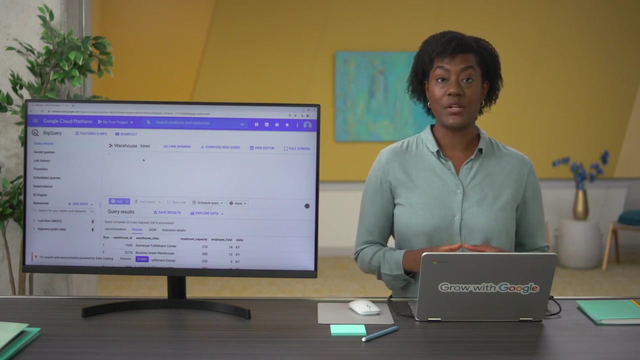 But let's check out an example to see count and count distinct in action. For this example, we're working with a company that manufactures socks. We have two tables, warehouse and orders. Let's take a quick look at these tables before we start querying. 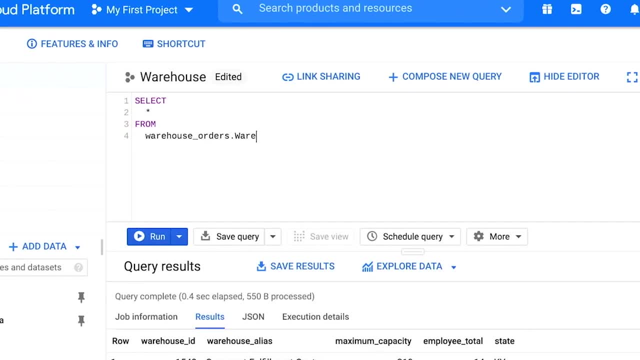 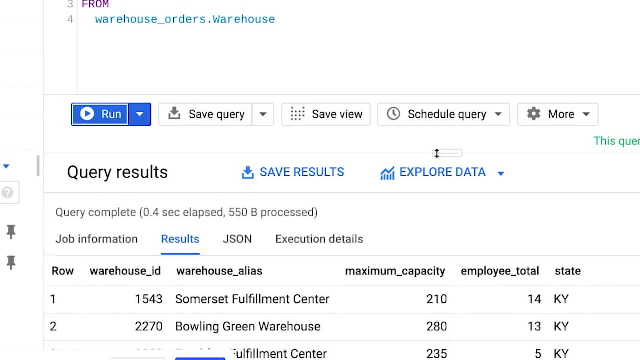 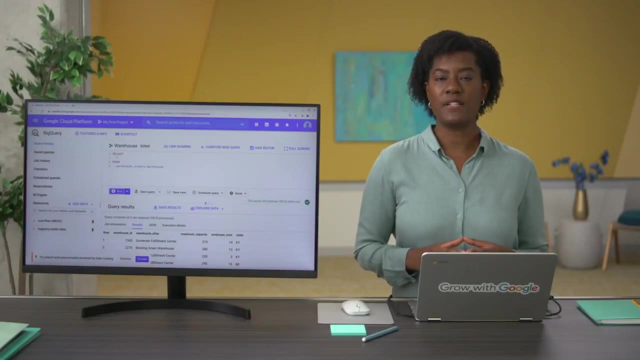 First we'll check out the warehouse table. You can see the columns here: Warehouse ID, warehouse, alias the maximum capacity, the total number of employees and the state the warehouse is located in. We'll pull up the top 100 rows of the orders table next. 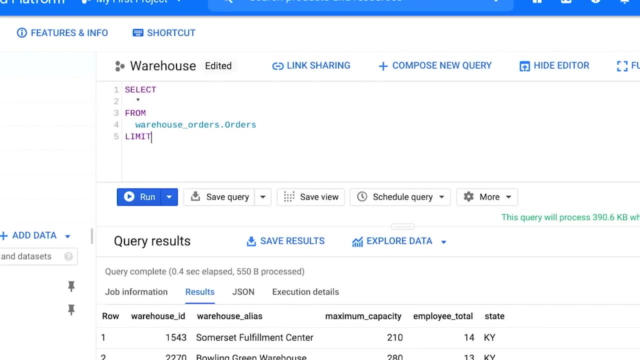 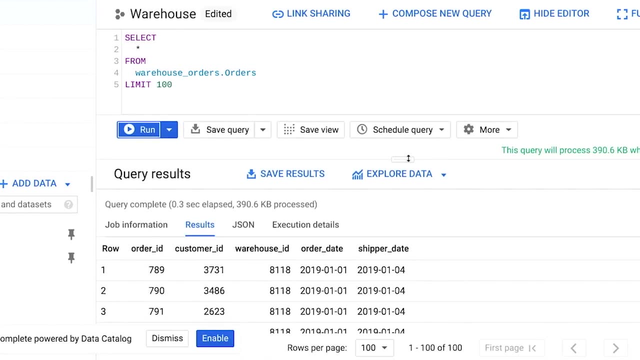 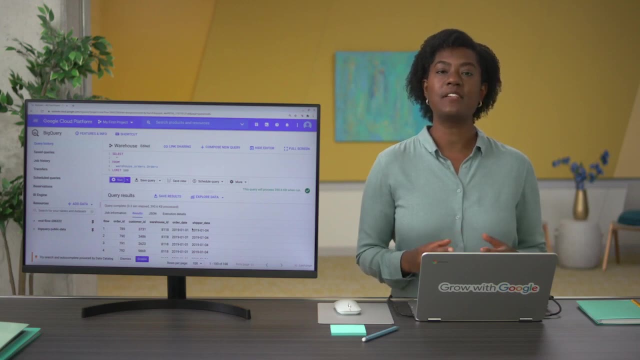 We can use limit here to limit the number of rows returned. This is useful if you're working with large data sets, especially if you just want to explore a small sample of that data set From this query. we're actually going to start with a from statement so that we can alias our tables. 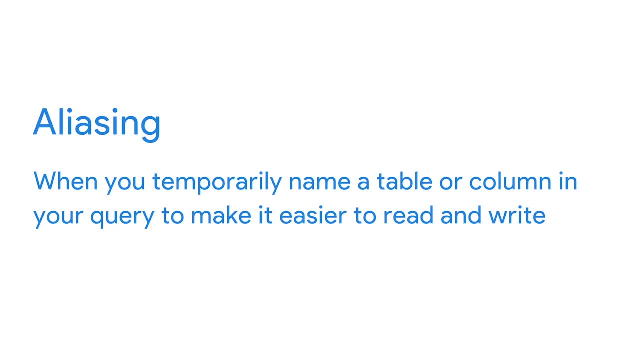 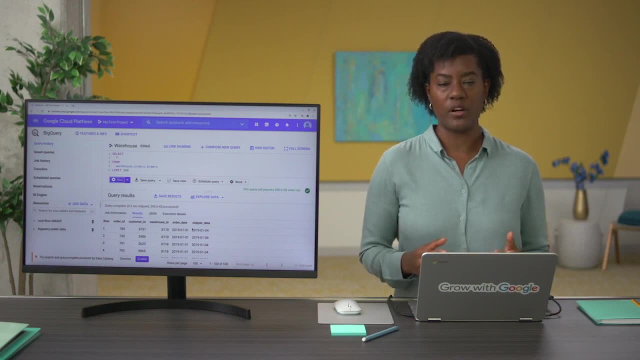 Aliasing is when you temporarily name a table or column in your query to make it easier to read and write. Because these names are temporary, they only last for the given query. We can use our from statement to write in what our tables' aliases are going to be. 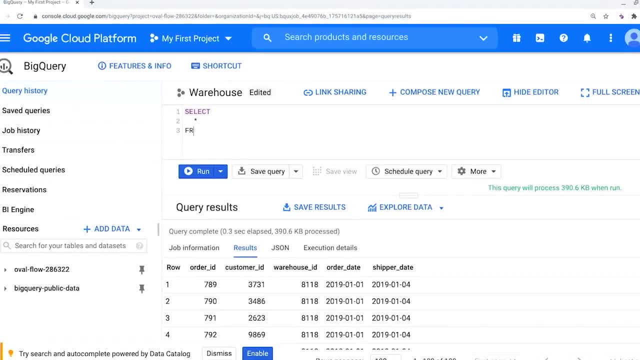 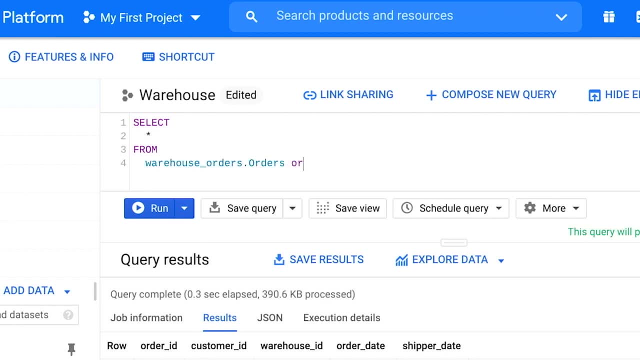 to save us some time in other parts of the query, So we'll start with from and use aliasing to name the warehouse orders table, just orders. Let's say we need both the warehouse details and the order details because we want to report on the distribution of orders by state. 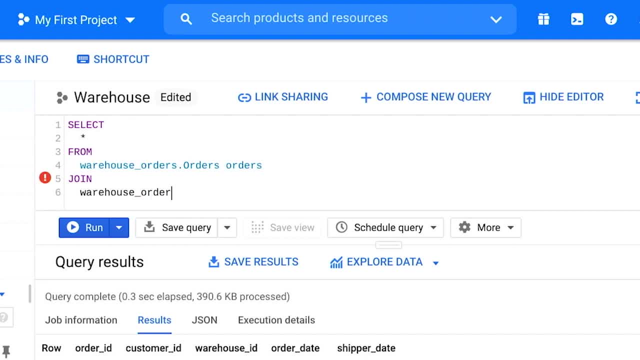 So we're going to join these two tables together, since we want data from both of them, and alias our warehouse table in the process. In this case, we're using join as shorthand for inner join, because we want corresponding data from both tables And now that we have the aliases in place, 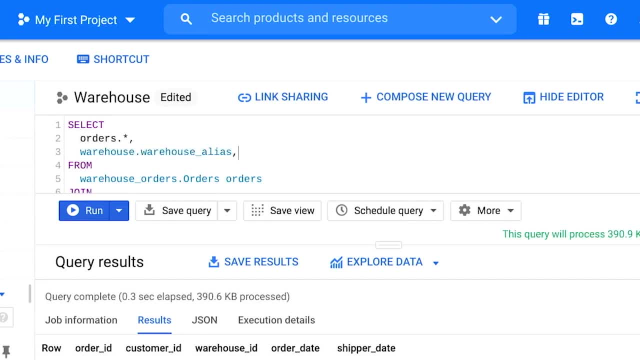 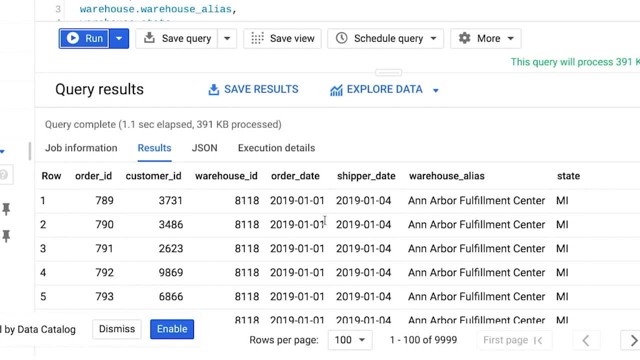 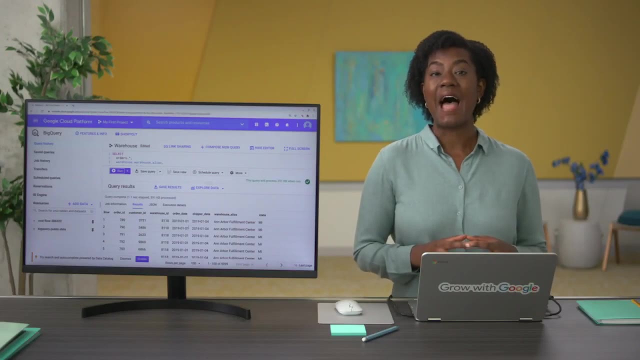 let's build out the SELECT statement that comes before from. Let's run that And there. Now we have data from both tables joined together and we know how to create these handy aliases. Now we want to count how many states are in our order data. 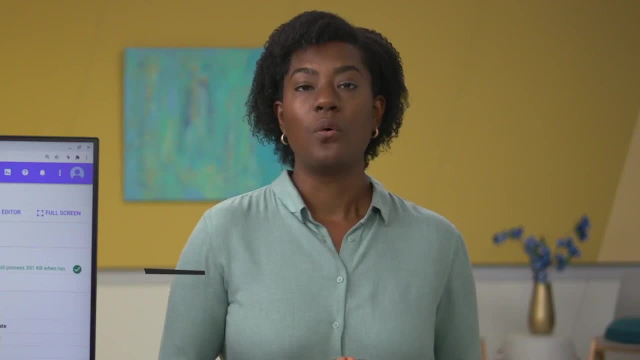 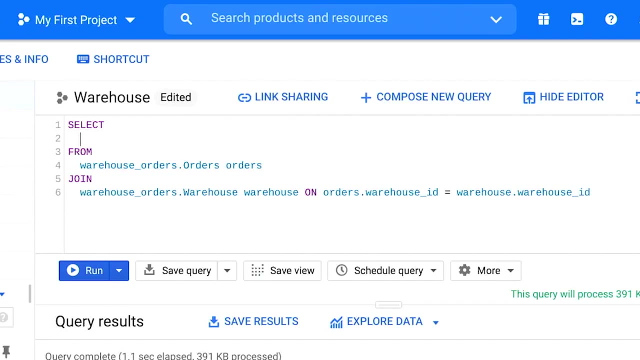 To do that, we'll use count and count distinct. now We can try a simple count query. first We'll join the orders and warehouse tables in our from statement And in this case we'll start with select and count the number of states. 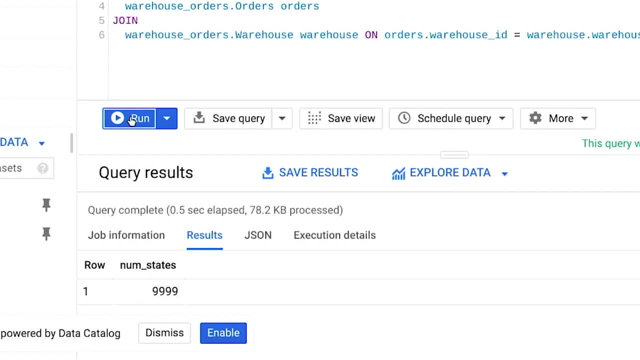 Let's run this query and see what we get. Wait, that's not quite right. This query returned over 9,000 states because we counted every single row that included a state, But we actually want to count the distinct states. Let's try this again with count distinct. 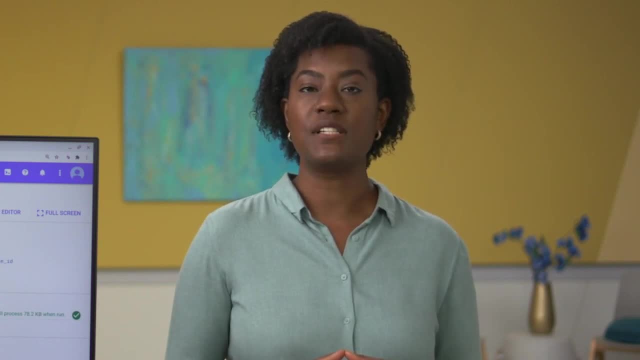 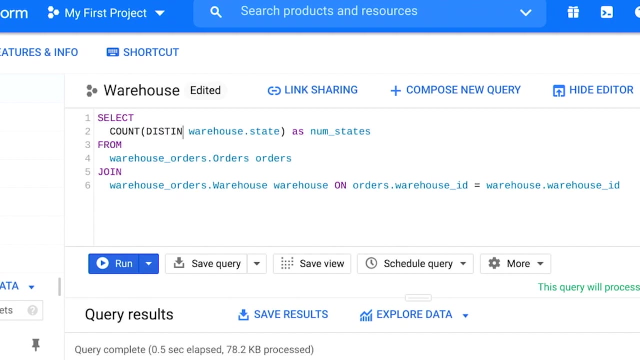 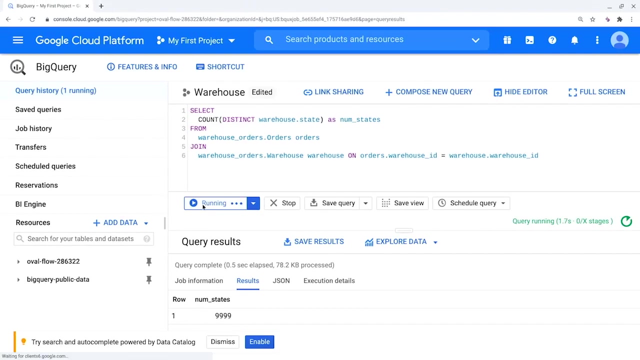 This query is going to look similar to the last one, but we'll use distinct to cut out the repeated instances that we got the last time. We'll use the query we just built but replace count with count distinct in our select statement. Let's try this query. 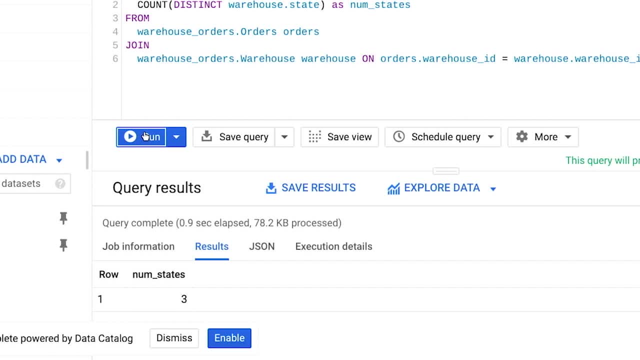 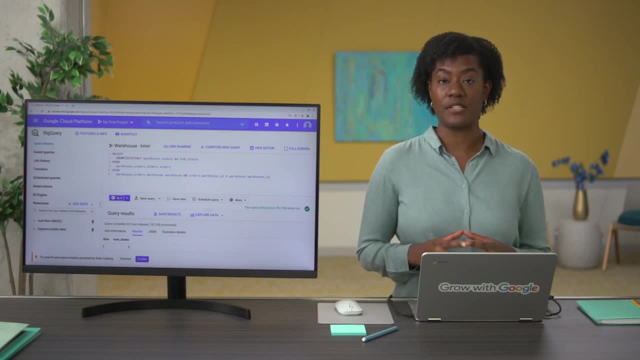 That's more like it. According to these results, we have three distinct states in our orders data. Let's check out what happens when we group by the state column in the warehouse table, which we'll call warehousestate. We'll use join and group by in our from statement. 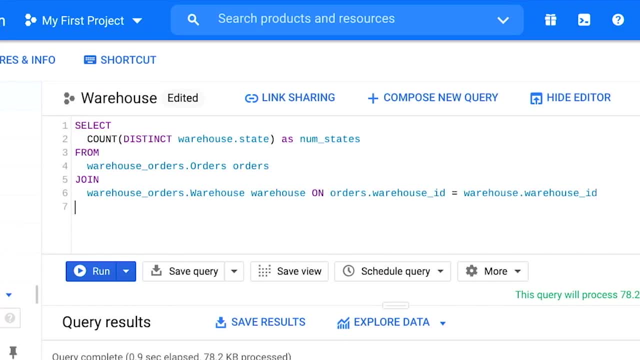 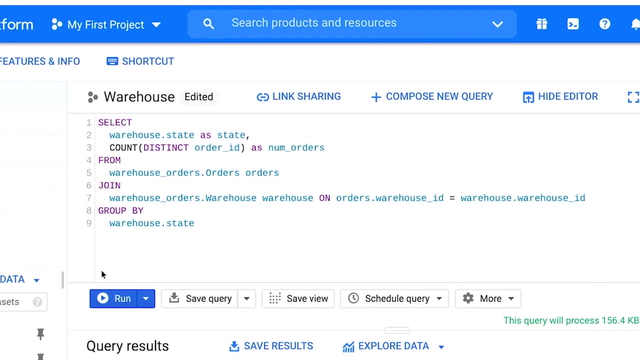 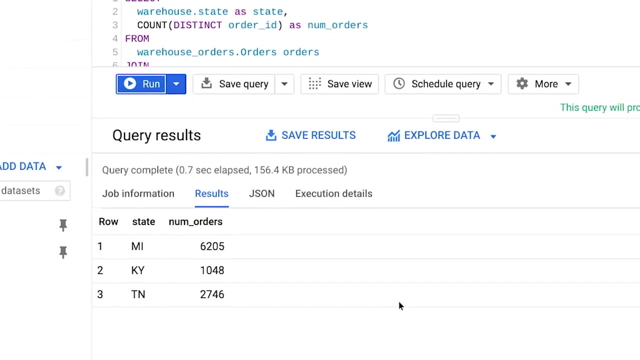 so let's start there again And then group by warehousestate. Now let's build out our select statement on top of that. We're still going to use count distinct, And let's run it Now. we have three rows, one of each state represented in the orders data. 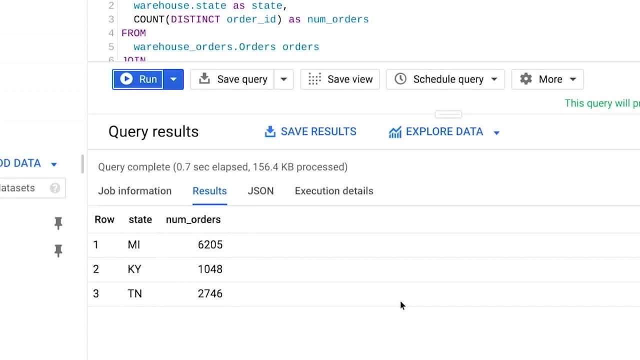 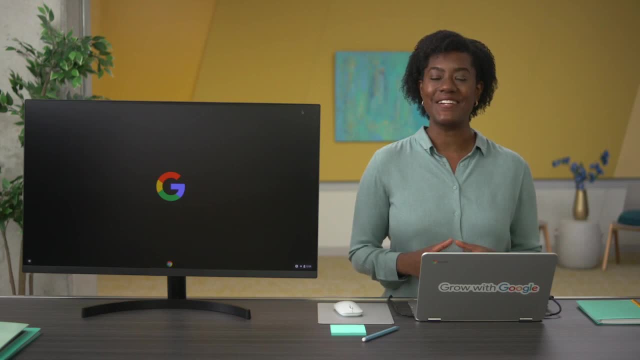 And our count distinct on the number of orders sums up the count we ran earlier: 9,999.. You'll find yourself using count and count distinct during every stage of the data analysis process, So understanding what these queries are and how they are different is key. 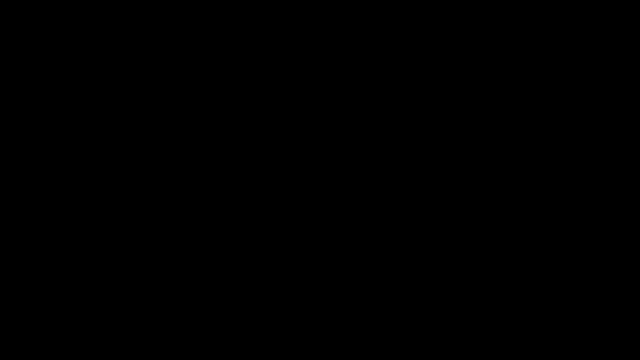 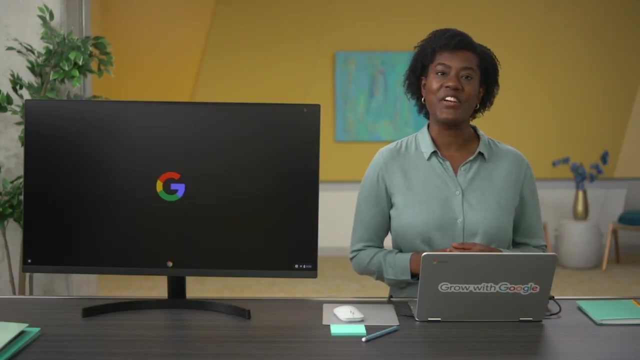 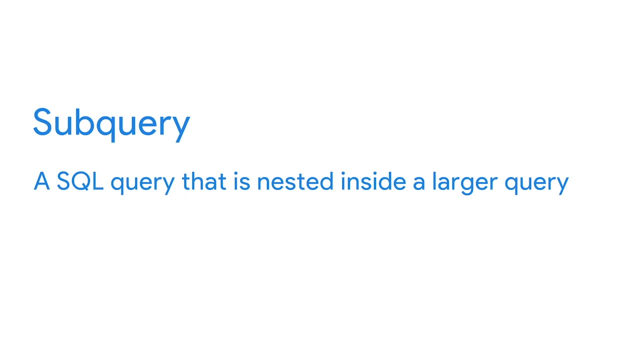 Great job and I'll see you again soon. In this video I'll introduce you to another kind of SQL query: subqueries. Your subquery is a SQL query that is nested inside a larger query. Have you ever seen one of those nesting doll toys? 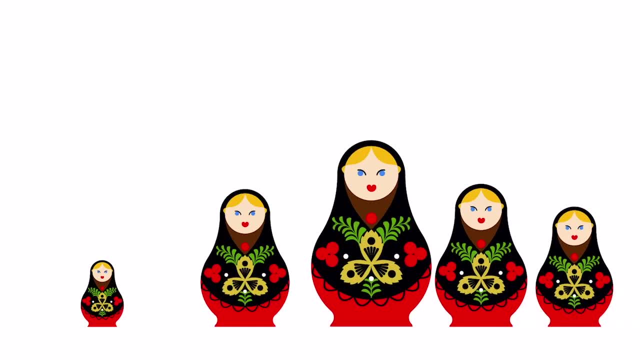 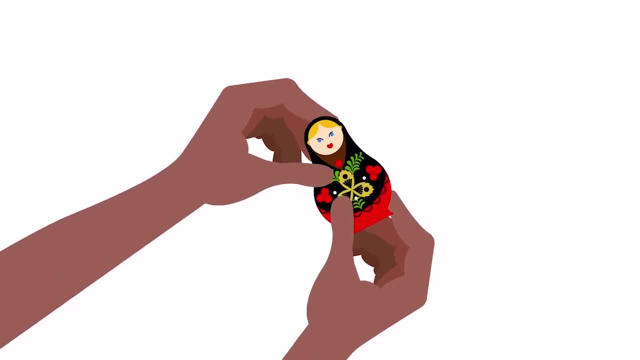 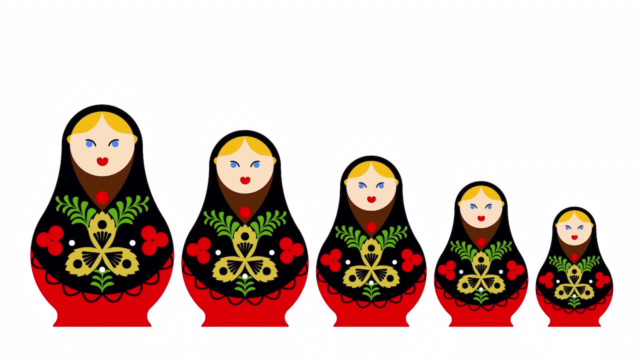 They're also known as matryoshku, Russian nesting dolls. Subqueries are a lot like nesting dolls. No, really. Your larger query could have a subquery in it, And then that subquery could have a subquery, And then that subquery could have another subquery. 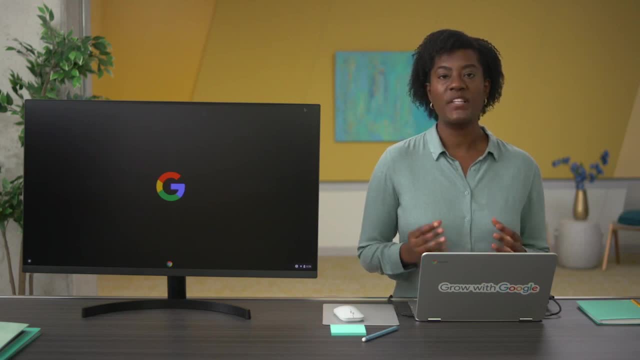 But when you stack them all together they make one query. With subqueries you can combine different pieces of logic together, Because the logic of your outer query relies on the inner query. you can get more done with a single query. This means all of the logic is in one place. 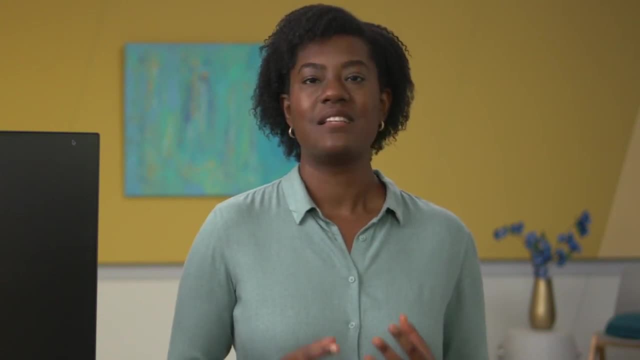 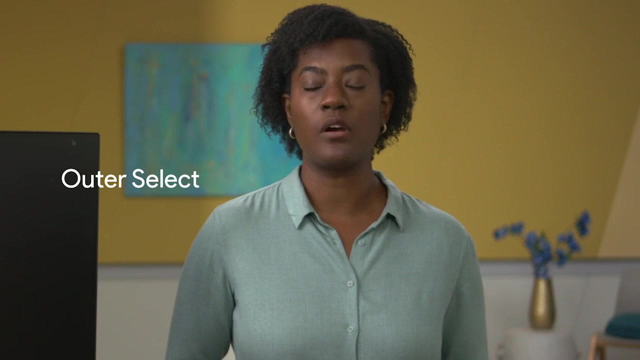 which makes it more efficient and easier to read. The statement containing the subquery can also be called the outer query or the outer select. This makes the subquery the inner query or inner select. The inner query executes first so that the results can be passed. 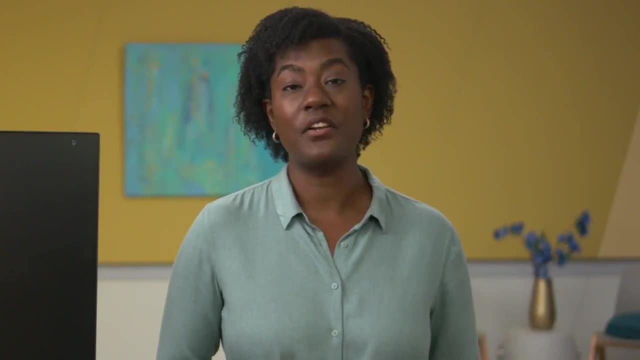 onto the outer query. to use Subqueries can get a little confusing because there's so many layers, But if you keep in mind that the innermost query executes first, it'll be easier to order your subqueries when you want them to execute. 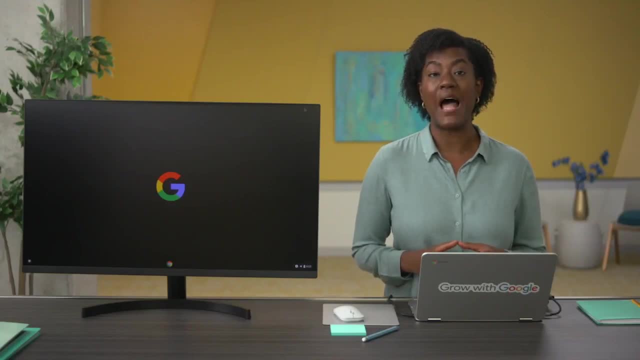 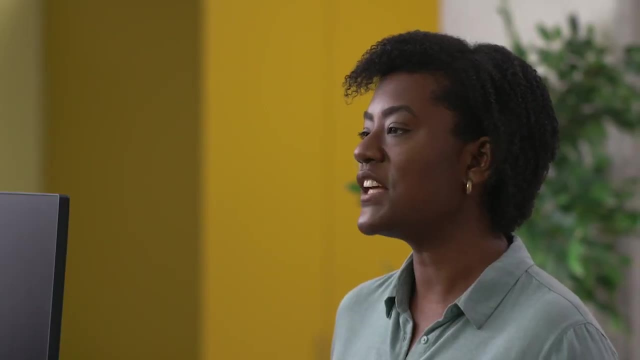 Subqueries can also be nested inside all sorts of other queries. Usually you'll find subqueries nested in from or where clauses. Let's try out some common subqueries. We'll start with a subquery and a select statement using the bike sharing data. 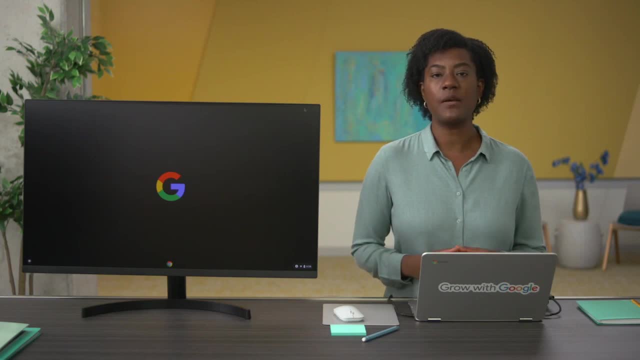 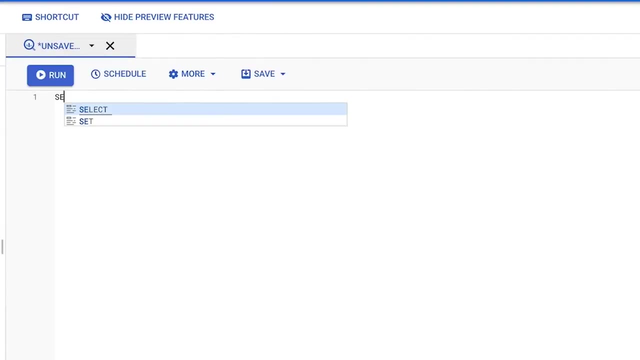 from an earlier example For the first statement. let's say we want to compare the number of bikes available at a station to the average number of bikes available. We're going to use this query to pull the average number of bikes available, Then we're going to incorporate it. 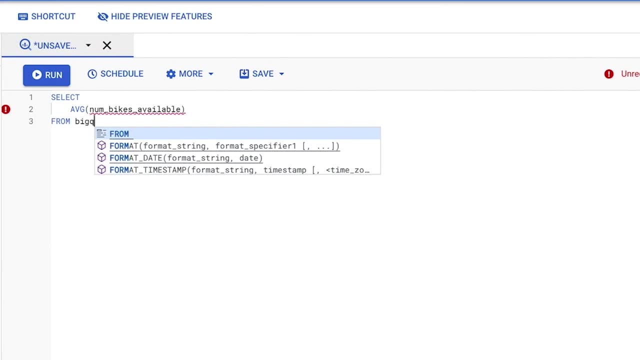 as a subquery. Now let's build our outer select query. We want to select the station ID and the number of bikes available. Then we'll put the select query- that's pulling the average number of bikes, inside that outer query by using parentheses. 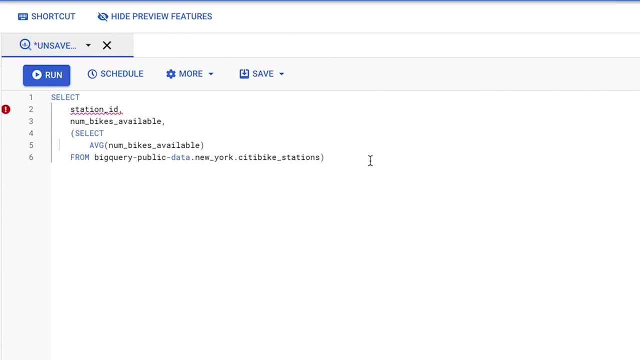 We'll also build from into the subquery before closing it with another parentheses And completing the outer query. The end of the outer join query has as to show what we want to call this column and a final from statement to indicate which table we're referring to. 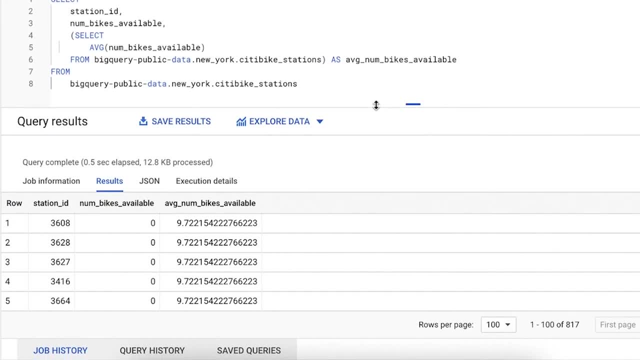 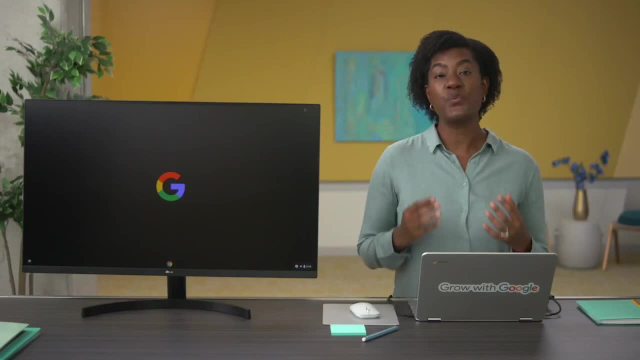 Now let's run it, And there we've got a table with both the number of bikes available and the average number of bikes available at different stations. It's really common to see subqueries nested in from and where statements, So let's try those next. 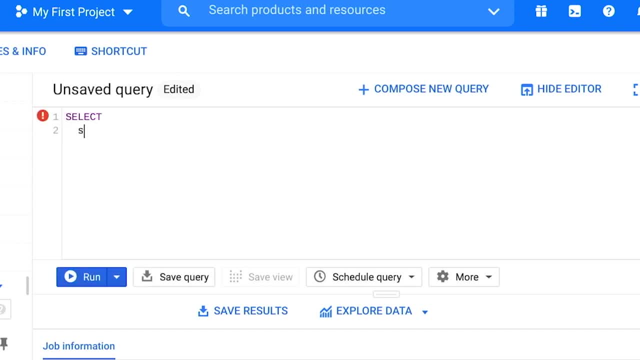 We could use a from statement to calculate the number of rides that have started at each station over time. We'll start with our outer query and input select station ID, name and number of rides. We'll use as to tell it how we want the table labeled. 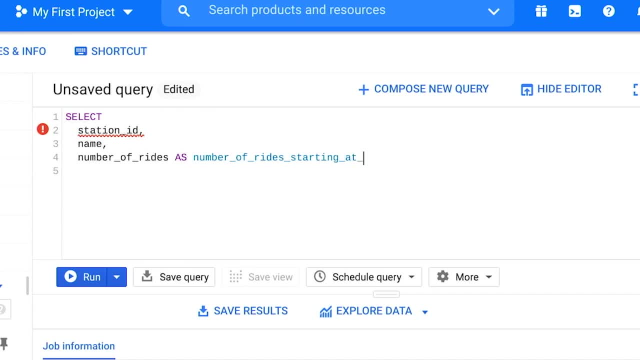 And from, to tell it where we're pulling data from. Before we finish that query, we'll add a subquery, We'll put our parentheses here and then select the start station ID. Then we can tell it to count the number of rides from the trip data. 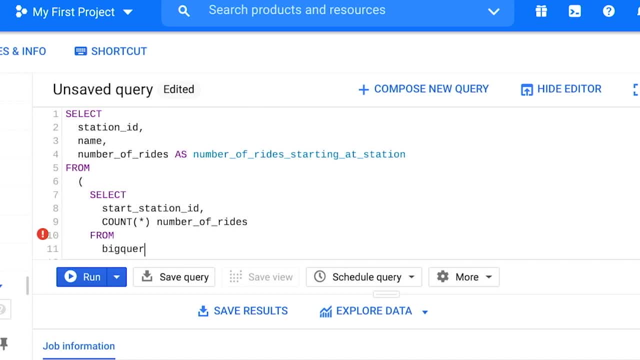 and group it by the start station ID. After that we'll close the subquery with a parentheses and continue building the outer query. We'll use as again, and then use inner join and on to join it with the station ID data And finally we'll tell it. 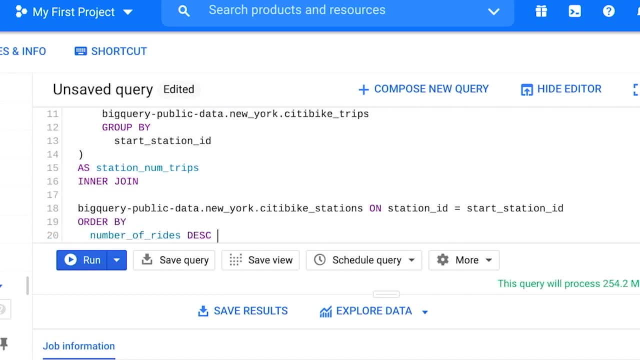 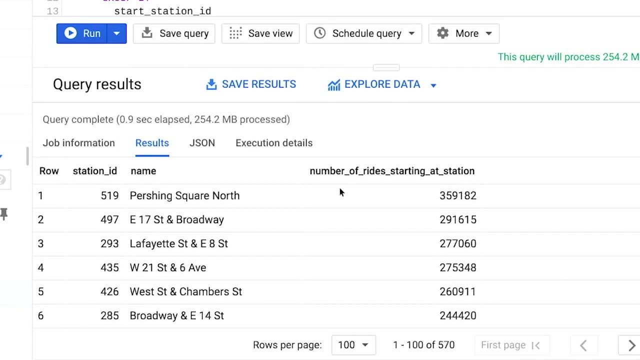 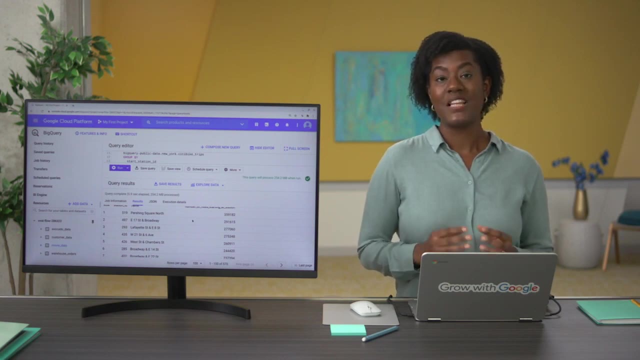 to put it in descending order. Let's see what happens when we run that. We now have the number of rides started at each station. Okay, One last example. Let's use a where statement. The bike sharing company has two kinds of users. 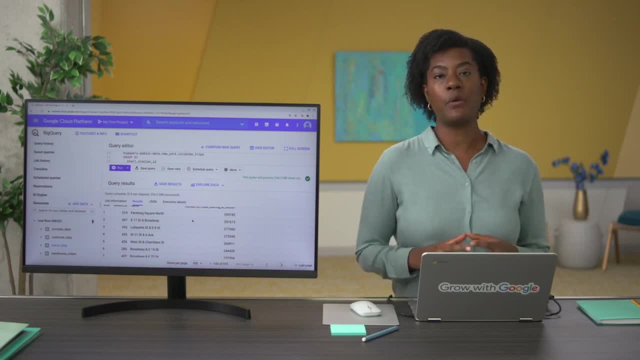 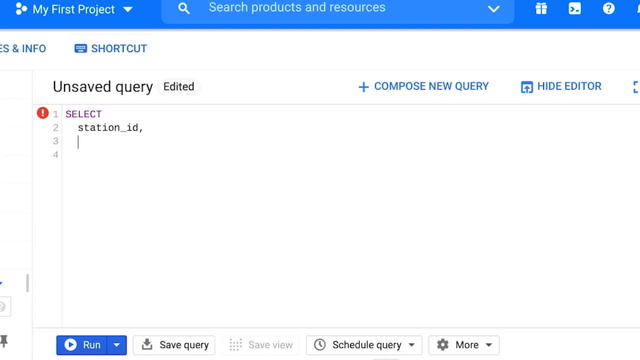 Subscribers and one-time customers. Let's say we wanted a list of stations subscribers used. As always, we start with the outer query, Select the station ID and name from the public data set we're using, And this time we'll use a where statement. 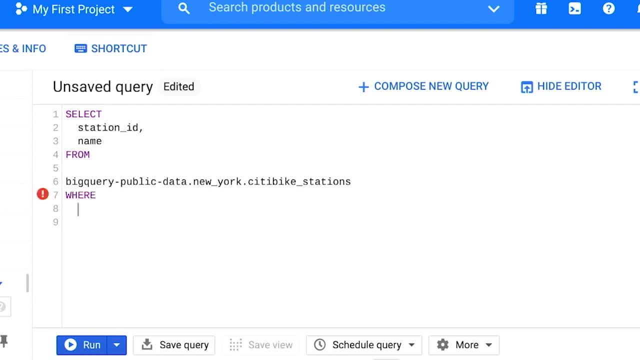 We'll also use in so that we can specify multiple values in this where statement. Then we'll put our subquery in the parentheses, We'll add select from and where again, But this time we'll tell it that we only want data on specific customers. 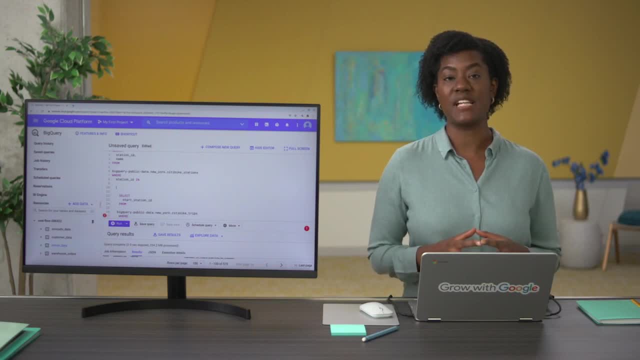 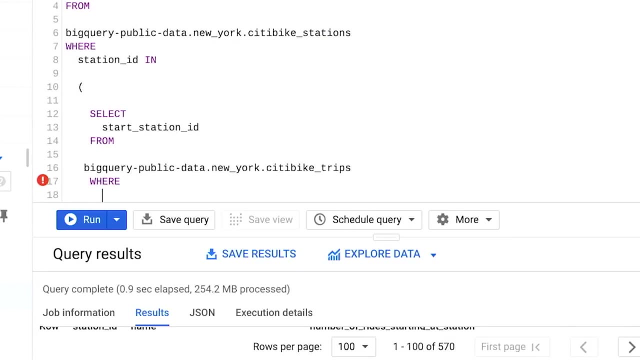 It's good to note that you can use comparison operators in subqueries, Even multiple row operators, like in any or all. In this case we'll use equals to indicate that we only want the subscriber user data. Now let's run the query. 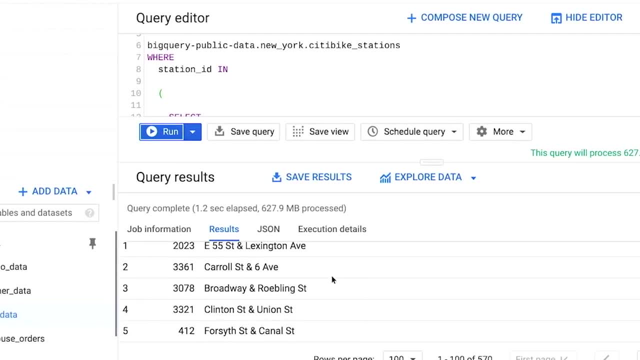 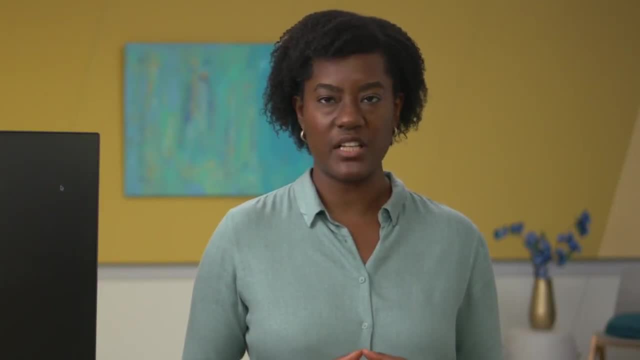 And we've got the station ID and names for stations that fit our criteria. So that's subqueries in action. Subqueries can be challenging. There's a lot of layers to think through And you might find yourself running into errors when you practice. 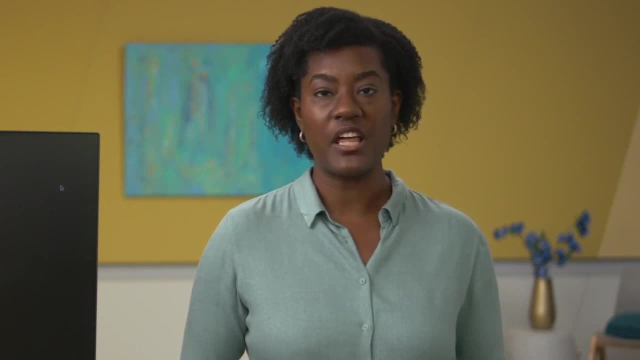 That's totally okay. Having to go through that challenge means you're growing. If everything was easy, we wouldn't find new ways to grow. For me, it's all about how much work and how much time I need to put in to do it. 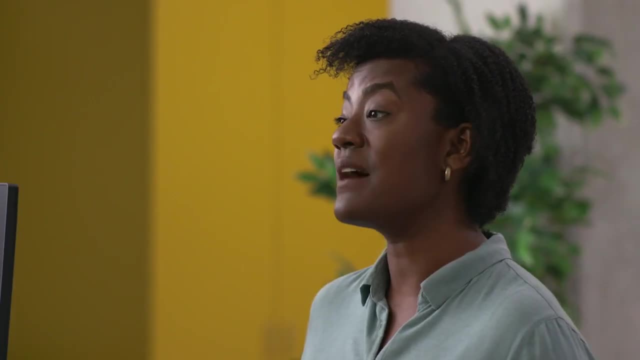 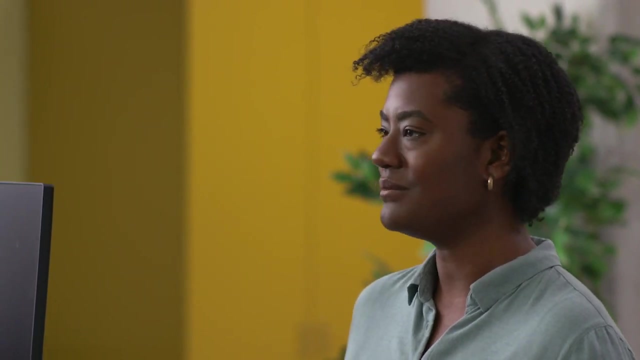 So give yourself time to practice this new concept Coming up. you'll get a chance to use subqueries to aggregate data or you can move on to the weekly challenge. You'll take everything you've learned, like using VLOOKUP, different joins and subqueries. 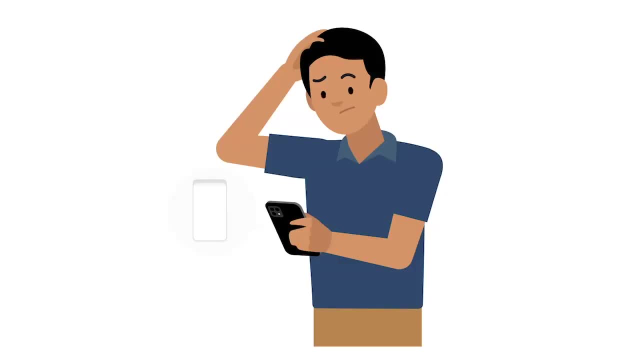 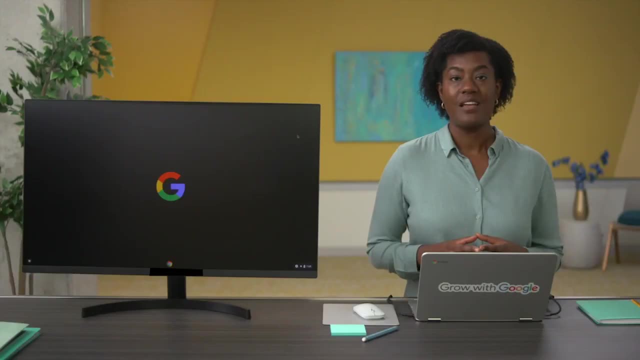 and apply it to this upcoming assessment. We've been doing a lot of complex work, So if you want to take a moment to review these videos before moving on, feel free, And once you finish the challenge, I'll see you again for our next big learning adventure. 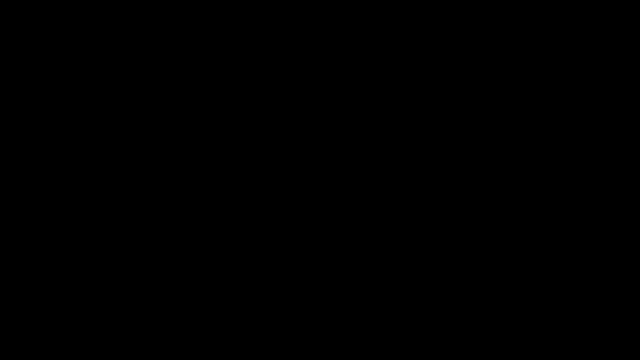 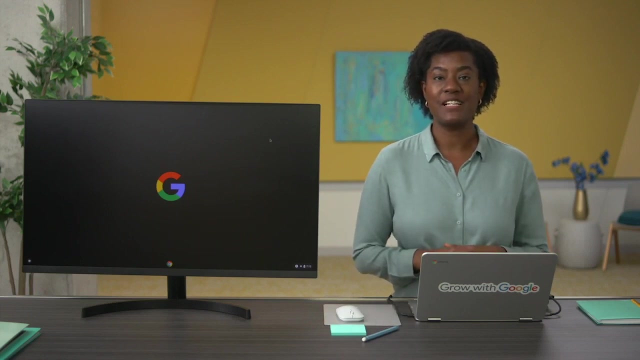 See you soon. Hey there, So we've got some experience nesting subqueries into our SQL statements to perform more complicated queries. Now it's time to talk about how to aggregate data. with subqueries Coming up, we'll learn about some new subquery statements. 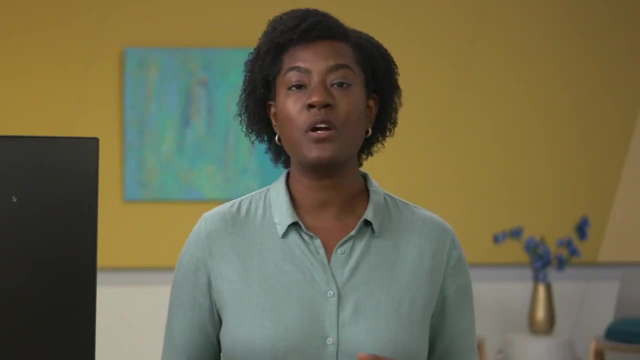 and use them to aggregate data. The query we're going to build in this video is pretty advanced. It's going to be a little complicated, but I know you've got what it takes. Let's get started. We've used functions like WHERE. 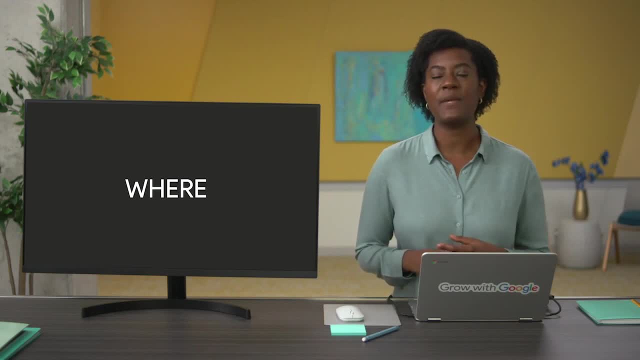 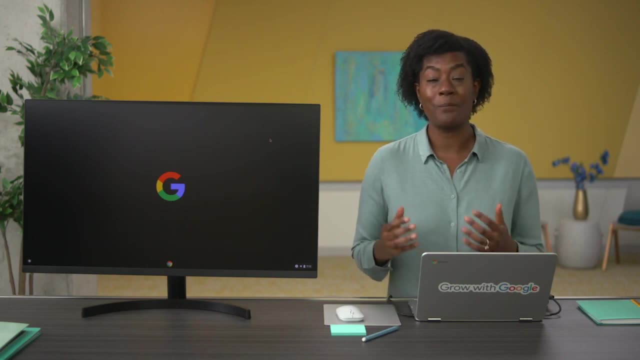 to filter our data before, but the WHERE function can't be used with aggregate functions. For example, you can use WHERE on a statement and follow it with GROUP BY, But when you want to use GROUP BY first and then use WHERE on that output. 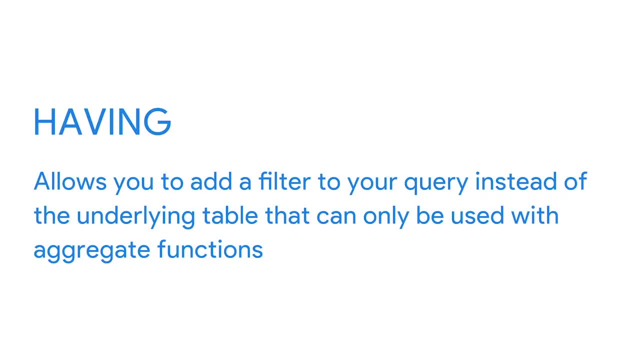 you'll need a different function. This is where HAVING comes in. HAVING basically allows you to add a filter to your query instead of the underlying table when you're working with aggregate functions. That way, it only returns records that meet your specific conditions. 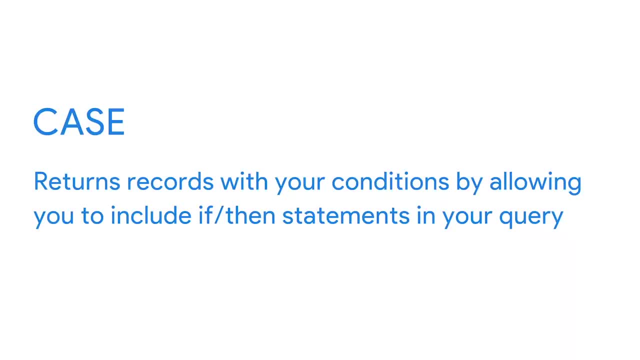 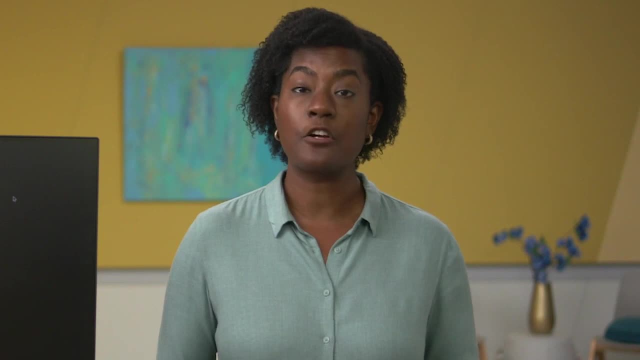 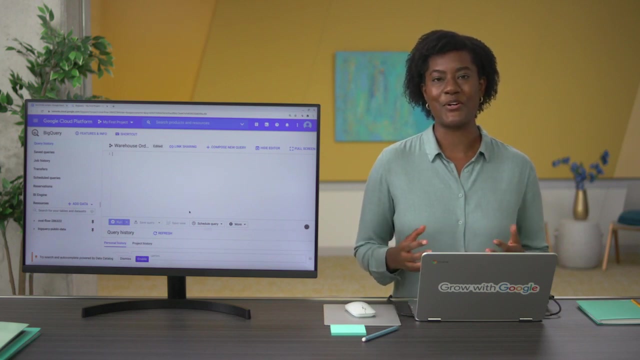 Similarly, CASE returns records with your conditions by allowing you to include IF slash THEN statements in your query. So let's try to aggregate our data with subqueries and test out these new functions. Let's say we're working with a company that makes socks that we talked about earlier. 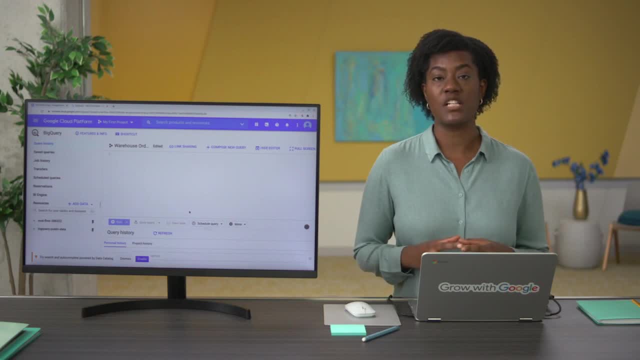 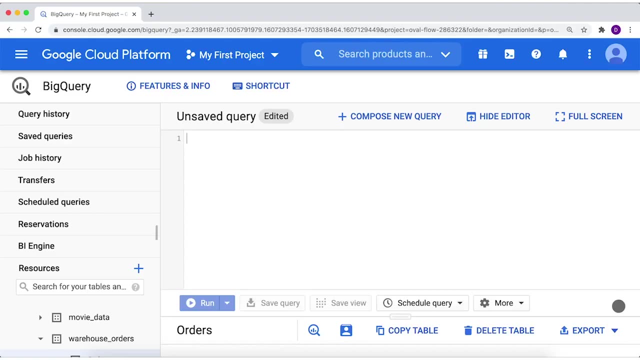 We've been asked to calculate what percentage of the orders are fulfilled by each warehouse. Basically, we're interested in knowing which warehouses are delivering the most orders. We've seen these tables before, but as a quick refresher, here's the orders table. 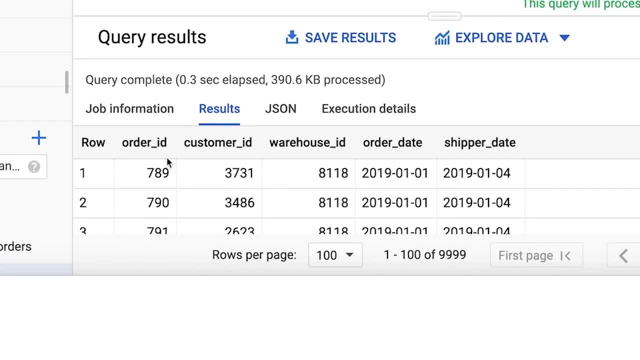 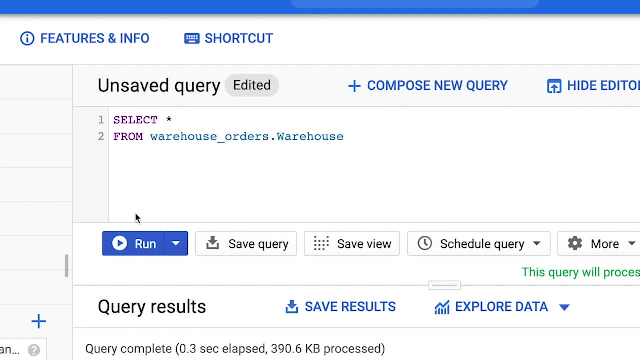 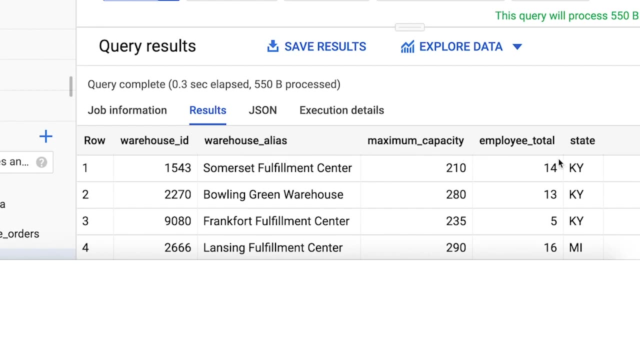 You can see the columns here: Order ID, Customer ID, Warehouse ID, Order Date and Ship Date. And if we pull up the Warehouse table we can check out its columns. We have the Warehouse ID, Warehouse Alias, the maximum capacity, the total number of employees. 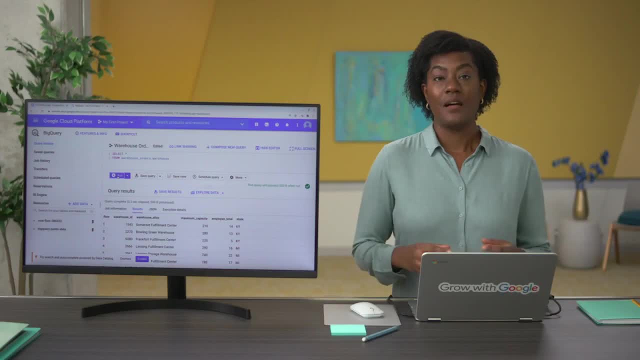 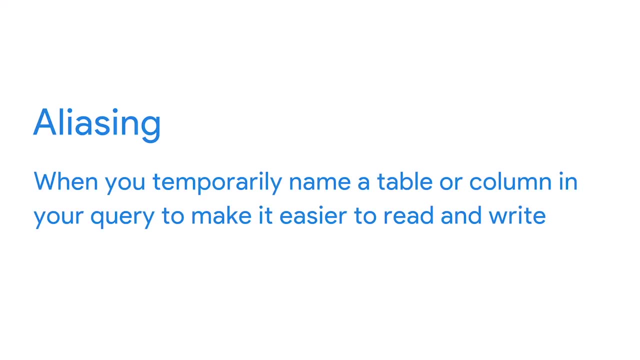 and the state where the warehouse is located. Before we start building the rest of our query, we'll want to alias our table names As a reminder. aliasing is when you temporarily name a table or column in your query to make it easier to read and write. 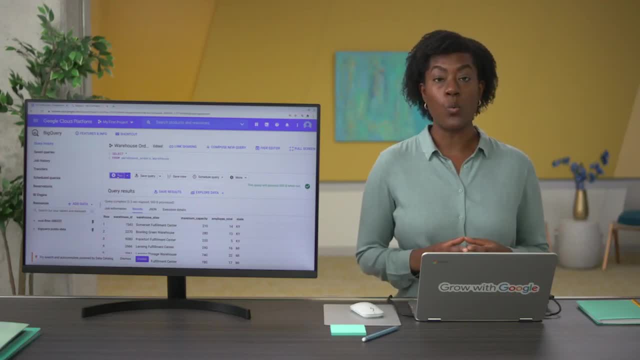 This example query is a little bit more complicated than the ones we've seen before, so aliasing will help save us some time. We'll start by aliasing the Warehouse table in our FROM statement. The FROM statement in this query is near the end. 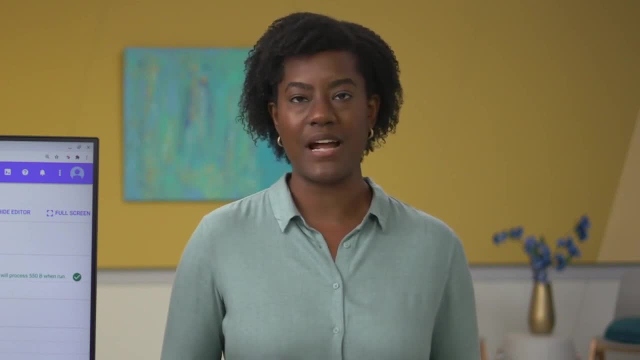 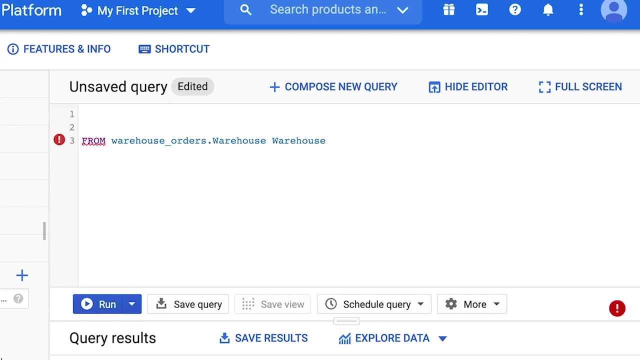 but we'll build this first so that we can use the alias everywhere else. We'll simplify it to just Warehouse. for the rest of this query, We know that we're going to join these tables together, so let's add that while we're working. 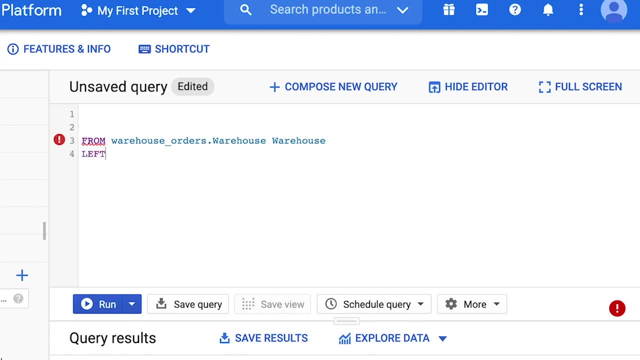 on this part of the query anyway. We're using a left join here because we want all the information from our Warehouse data, even if it doesn't show up in the ORDERS table. Then we'll alias the ORDERS table as part of this statement. 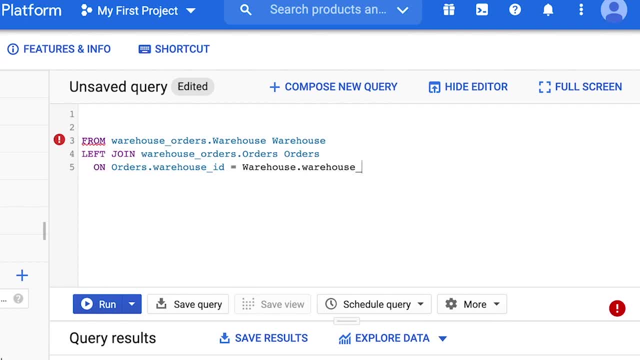 Now both of our tables have temporary names we can use and we've already finished a join statement. But before we can build the beginning of this query, let's go ahead and add our GROUP BY statement. after this join, We'll group these by the Warehouse ID and name. 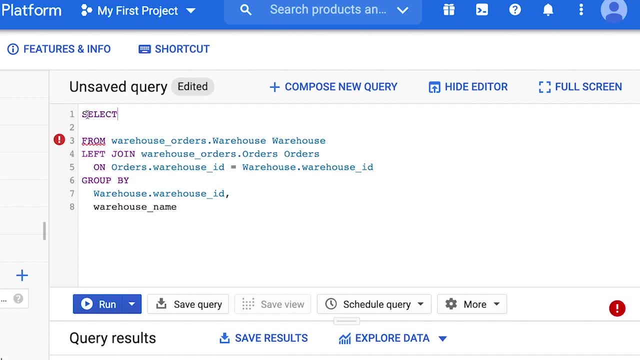 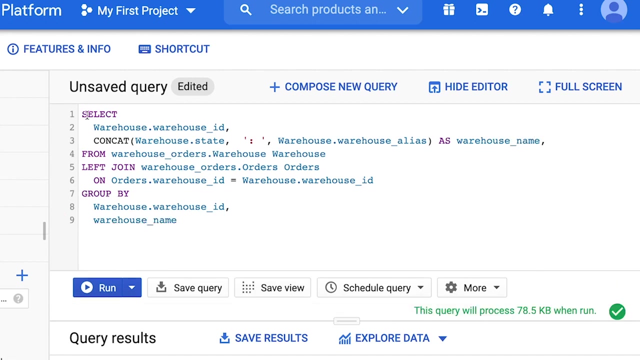 And now we'll go back to the beginning of the query. We'll select the Warehouse ID, Then we'll use CONCAT to combine the strings with the Warehouse's state and alias as the Warehouse name. Then we'll use COUNT to get the number of orders. 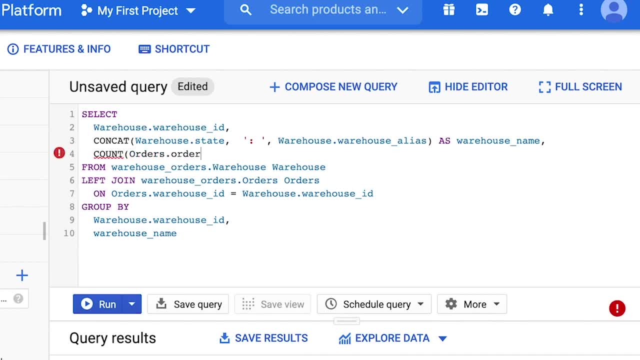 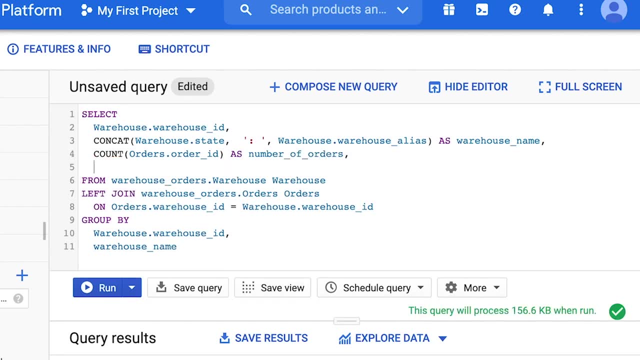 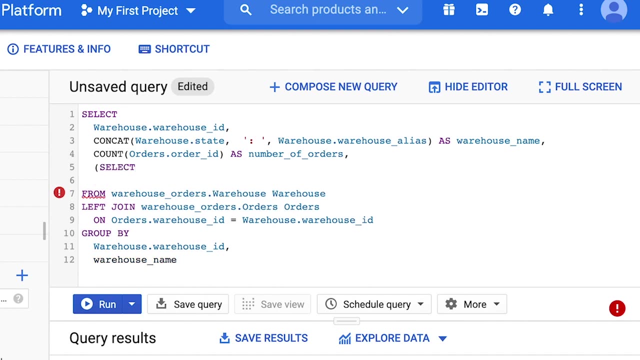 per Warehouse. Next, we'll build in a subquery to pull the total number of orders placed across all Warehouses. We'll input SELECT again and then write the subquery in parentheses. We'll put an asterisk after COUNT to indicate that we want to include everything from the ORDERS table. 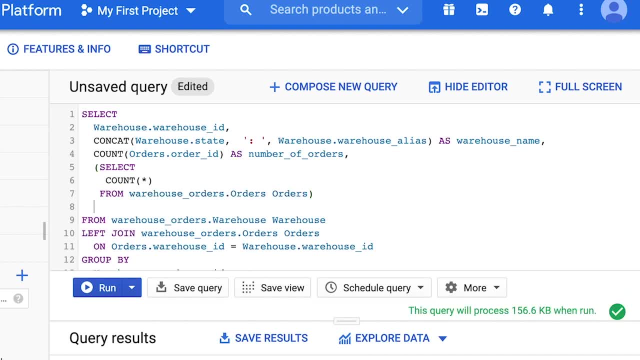 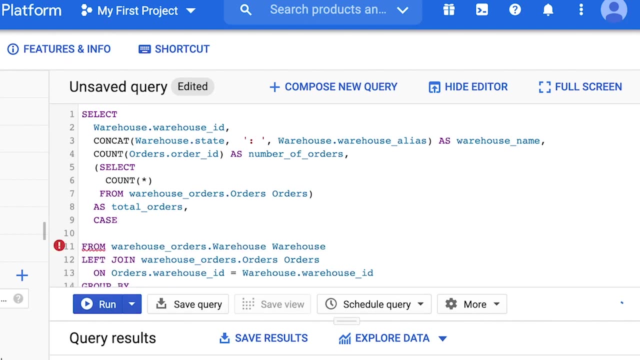 And finally, we'll close out the subquery and use AS to name this column: Total Orders. Now that our subquery logic is complete, we can use a CASE statement to create categories for our Warehouses based on how many orders they will fulfill. 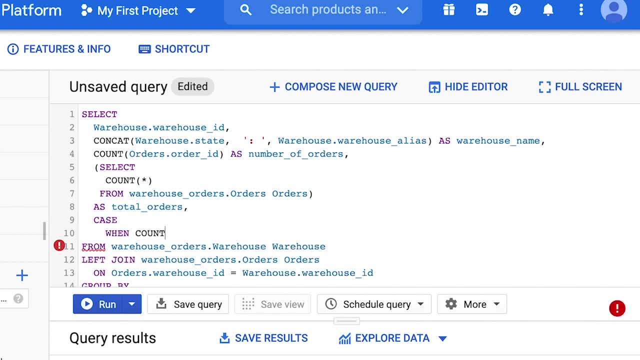 We'll represent these as percentages. You should notice COUNT in this statement a few times. We'll start by saying when the number of orders from our ORDER table is less than or equal to 0.2.. Then the table will say FULFILLED: 0-20%. 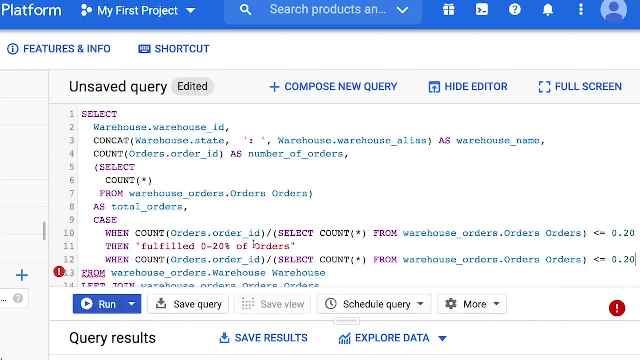 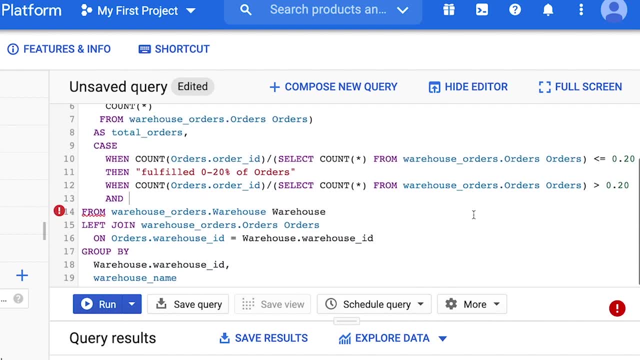 of ORDERS, And then we'll use WHEN again to indicate that when the number of ORDERS is greater than 0.2 and less than or equal to 0.6, it'll say FULFILLED 21-60% of ORDERS. 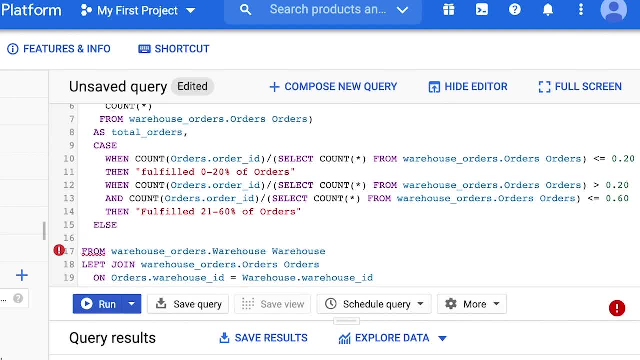 After that we can use ELSE to have everything that doesn't meet the criteria of our CASE statement, say FULFILLED more than 60% of ORDERS. Then we'll use END AS to name this column: FULFILLMENT SUMMARY. 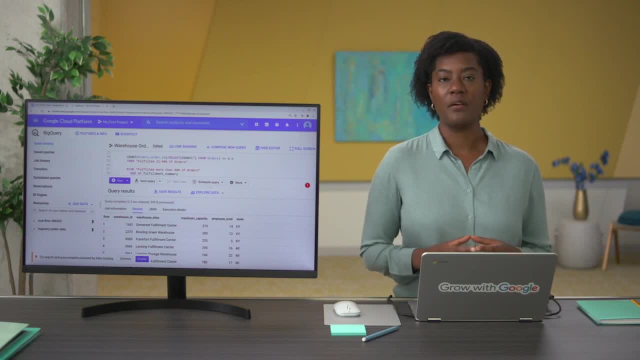 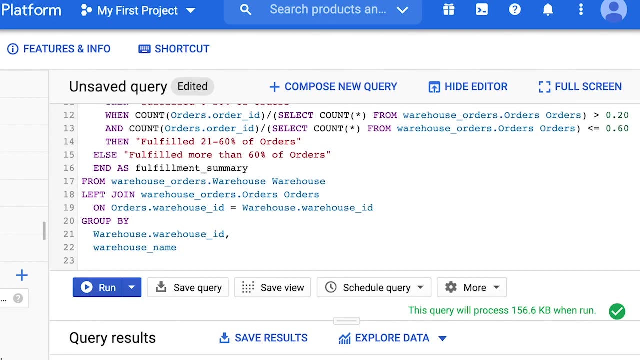 That brings us back to the portion of the query we've already written, but we're going to add a HAVING statement at the very end of this query. Our Warehouse table has warehouses that are currently being built and we want to filter those out, since they aren't fulfilling orders yet. 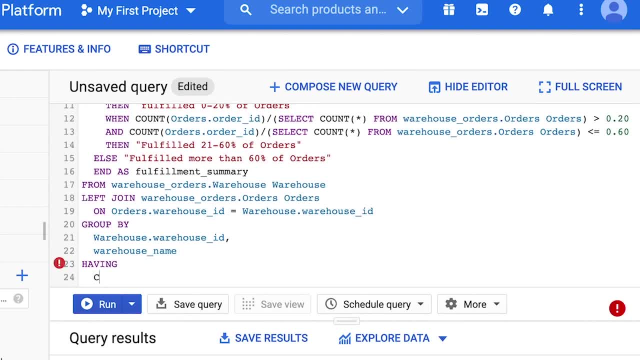 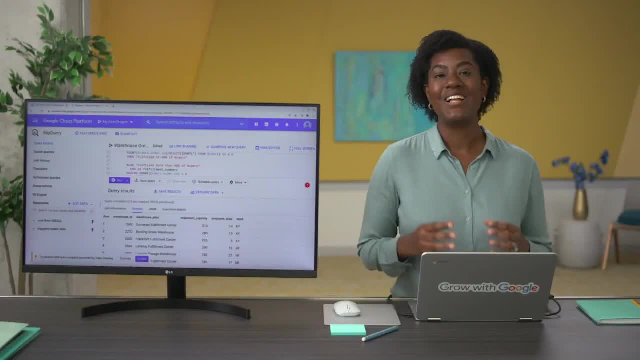 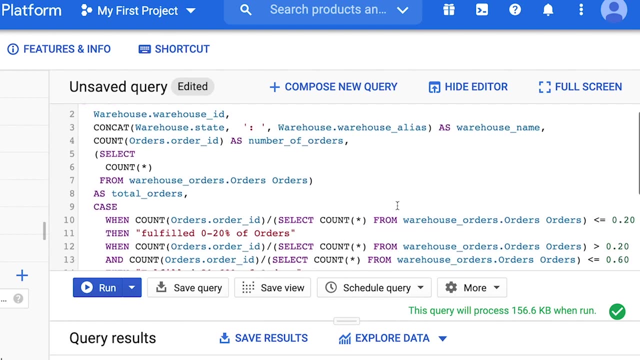 We can use HAVING to only include warehouses that have at least one order. Now, before we execute this query, let's take a moment to look at the whole thing. We have an OUTER SELECT, a COUNT subquery, a CASE statement, a JOIN and HAVING. 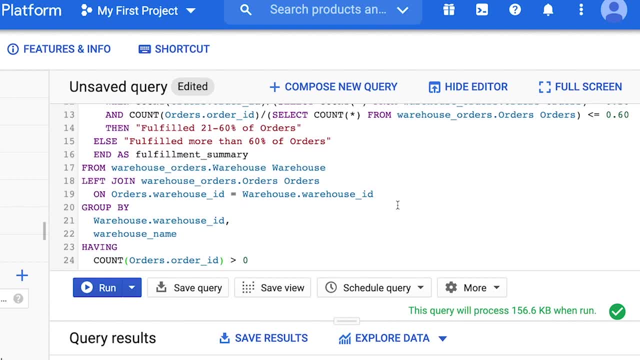 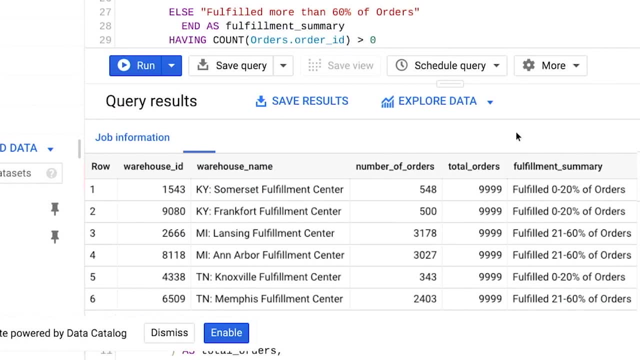 all wrapped into one query. We've built a really complex query, so let's run it to see the new table, And there Now we can easily identify what percent of our company's total orders are being fulfilled by each warehouse. These warehouses met our criteria. 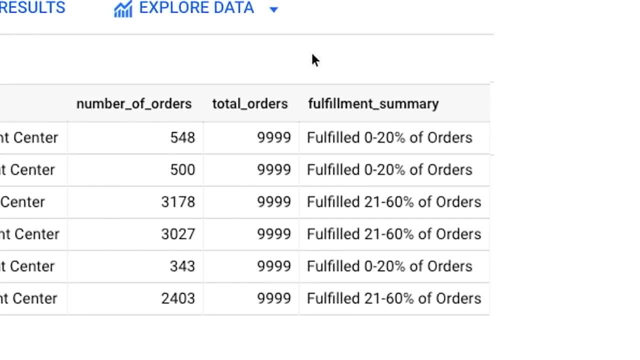 and we can see here in the FULFILLMENT SUMMARY column the percentage categories we outlined in our CASE statement. Obviously, since we included a HAVING statement to specify only warehouses with at least one order, there aren't any warehouses currently under construction. 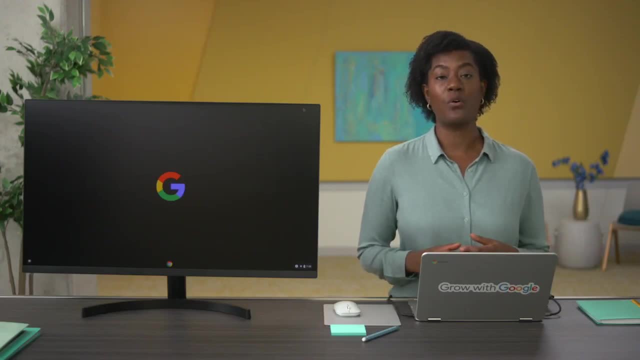 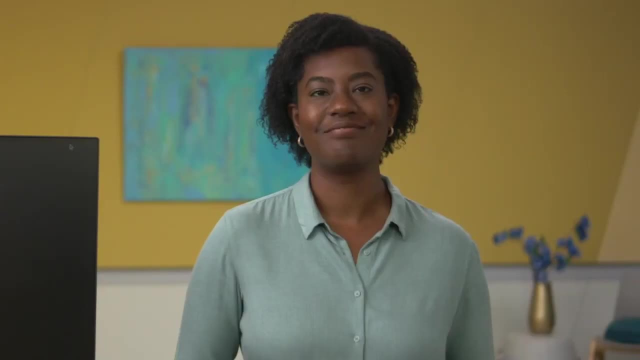 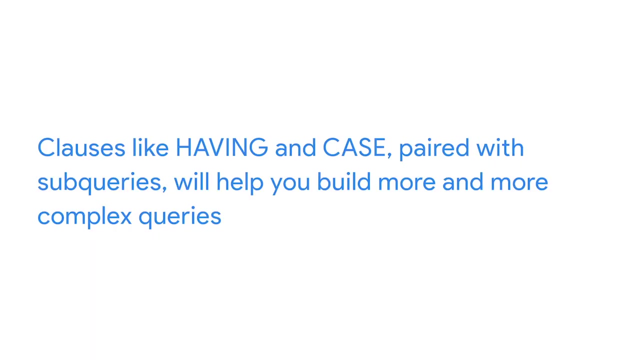 in this table. That really complicated query created this specific table of data we can use to easily compare how these warehouses are performing. There you go. That's a quick taste of what it's like to work with subqueries and data aggregation Clauses like HAVING and CASE. 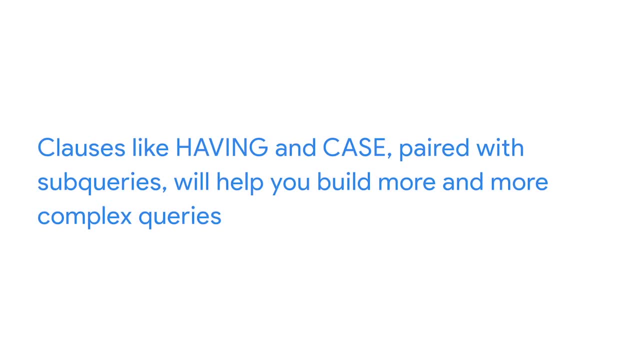 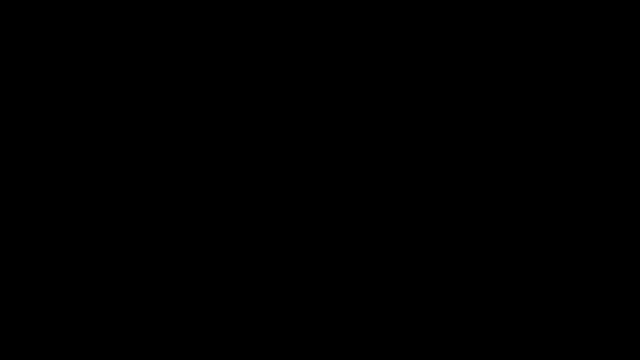 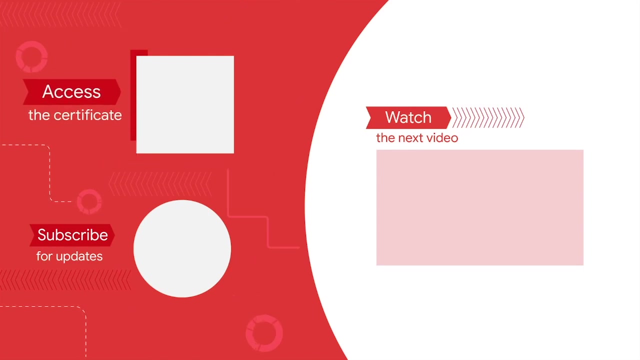 paired with subqueries will help you build more and more complex queries, which lets you do more and more complex things in SQL. Congratulations on finishing this video from the Google Data Analytics Certificate. Access the full experience, including job search help, and start to earn the official certificate. 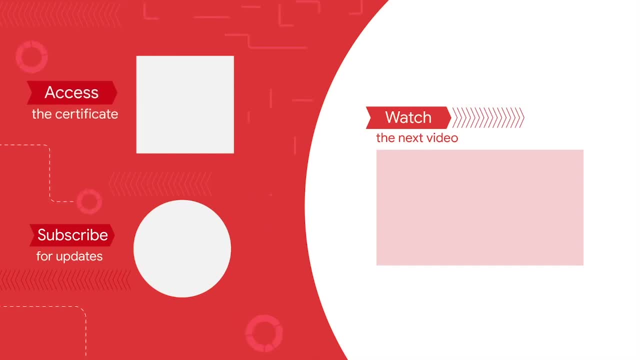 by clicking the icon or the link in the description. Watch the next video in the course by clicking here And subscribe to our channel for more from upcoming Google Career Certificates.